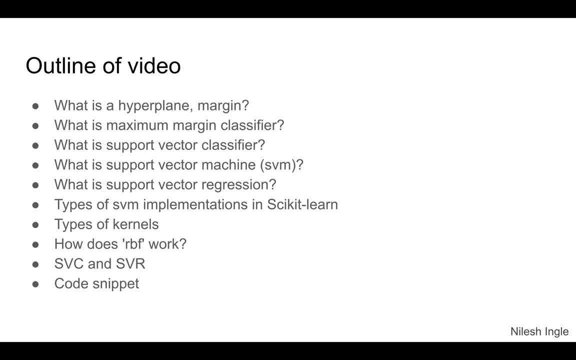 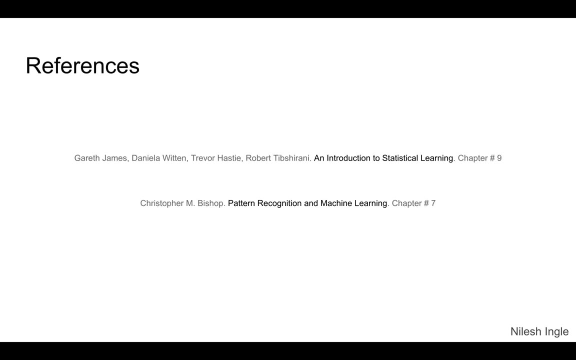 uh, roughly these topics hyperplane. what is maximum margin classifier? uh, then support vector classifier, support vector machine, etc. and see how the, how, this intuition all plays out in this video. for references, i've listed two references here. uh, one is the introduction to statistical learning, chapter 9 and chapter 7 from pattern recognition and machine learning. 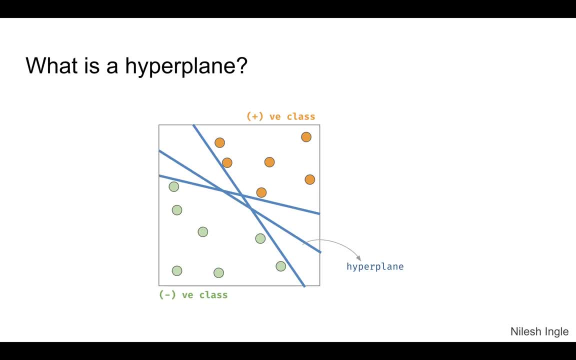 so what is a hyperplane? uh, so, as we can imagine, on this particular plot, let's say we have these, uh, orange data points and we have some green data points that we need to separate these two classes so we can draw lines, straight lines through each of. 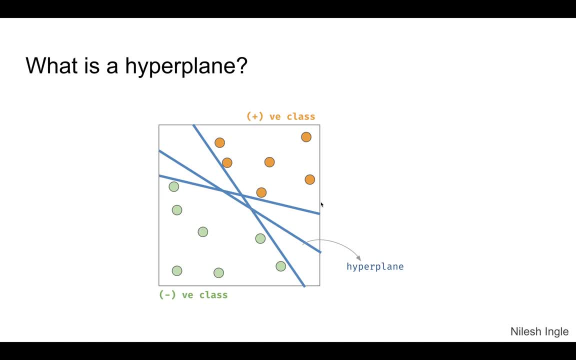 through this plot so that we can separate this. so here are three lines that we can draw and there could be infinite number of lines, so each of these lines that we are drawing here could be called as a hyperplane. so in general, the dimensions is one less than the dimension of the data set. so if we have here, we have a two-dimensional data set. 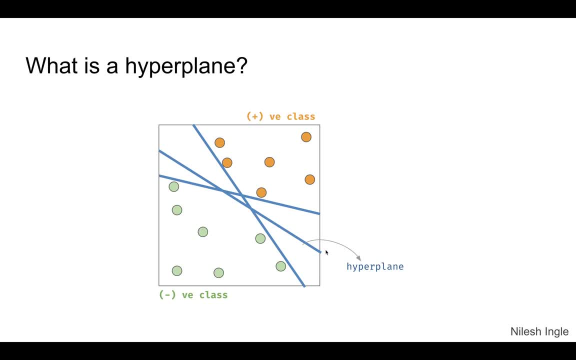 so the hyperplane would be one dimensional and hence the line: if it's a three-dimensional data set, hyperplane would be a two-dimensional plane. then what is a margin? now, a margin is, uh, as shown here in this particular plot. let's say: this is the decision boundary we have. 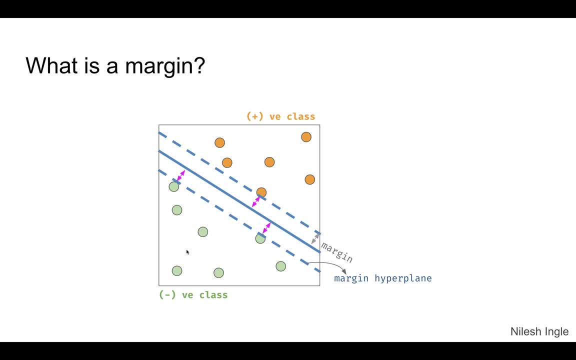 a solid line that separates the orange data points from the green data points, and then we look at the closest data point on of each of those two classes to the decision boundary. so in this case, this particular point is closest to the decision boundary and on this side, these: 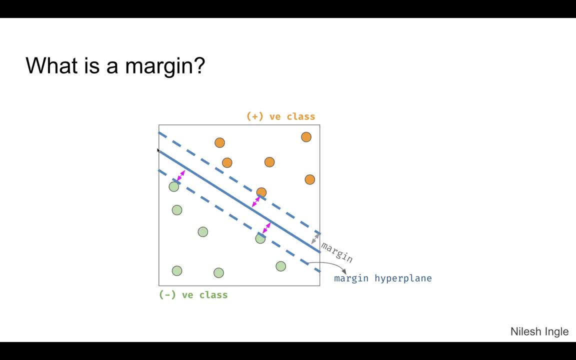 two are the ones that are the closest one. so the middle ground, so the that we can draw between those two, between these sets of closest point right through the middle, uh, will divide the space into two, and so each of the space is shown here by magenta arrows, and those are the margins, and the dotted line then is the, again the margin. 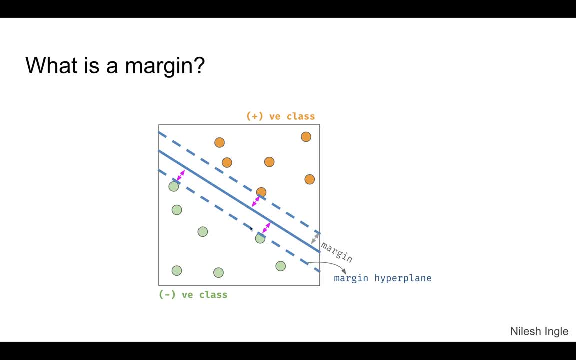 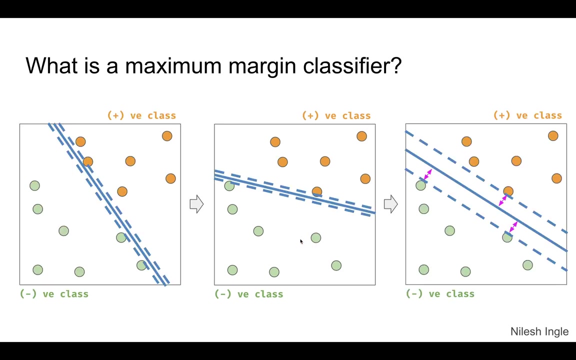 hyperplane, or that is also a decision that could be thought of as a soft margin, as we'll talk later on. so margin is, uh, uh, nothing but this space that's around, uh, the main solid decision boundary that we have. so what's the intuition behind the maximum margin, classifiers? and so, as we saw before, we 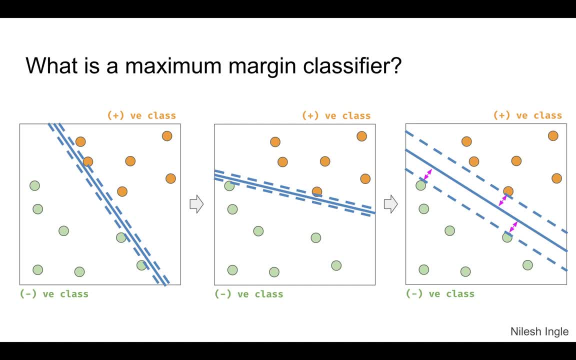 could draw hyperplanes in various uh positions. and so if you draw hyperplanes, as shown in this particular case, the leftmost figure- we see that the margin is there, uh, which is a very narrow margin, uh, because the dotted lines are very close to the solid line. same thing in the 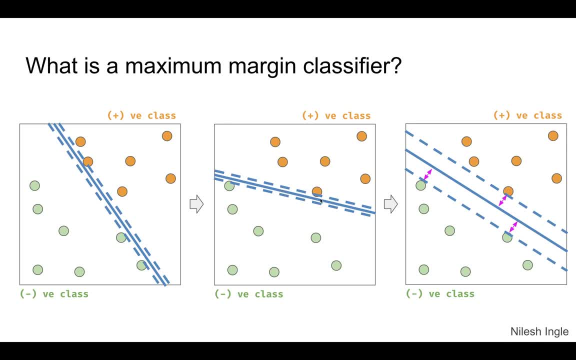 middle figure. we do have the separation of classes, but then the margin is too tight. so the solid line is very close to the dotted lines there. and what happens in this case is if there are new data points, margin has to shift drastically to accommodate that new data point to the correct class. 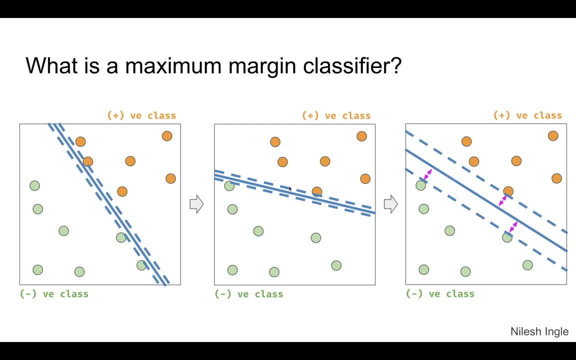 and so the another idea then is to generalize, to be to have ability to generalize more to a new data set. what we want is a margin that that is such that it's we can get the maximum space between, maximum space of separation between the two classes. so if we look at these- the figure on the 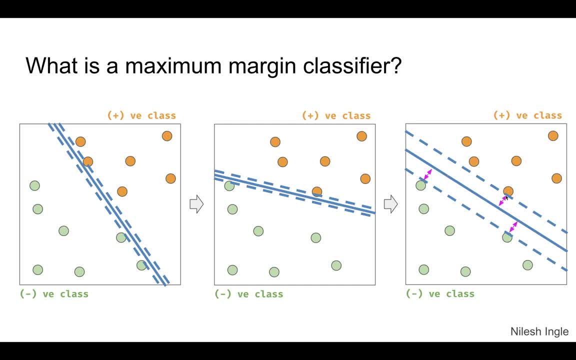 right. we see that this is the max. we get a maximum separation between the two classes if you draw this solid line right through the middle of these, these two green dots and this one orange dot, and so we do have the dotted line shifted far away from the solid line, and thus we can 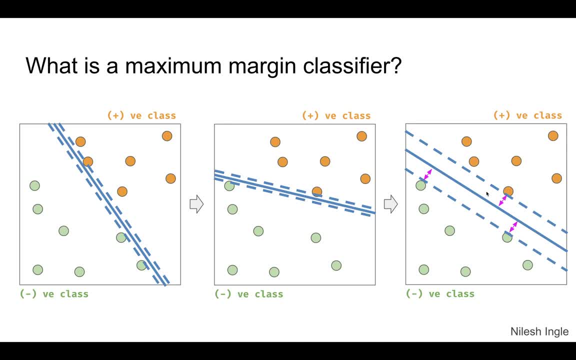 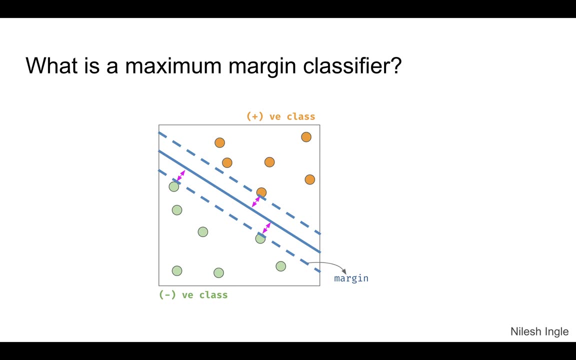 in this position we get the maximum width or maximum margin, and so the classifier that tries to classify data points using this approach is called as the maximum margin classifier, and again in maximum margin classifier, as we saw this can be. this idea of maximum margin can be built up more on what is called as a support vector classifier, so in support vector. 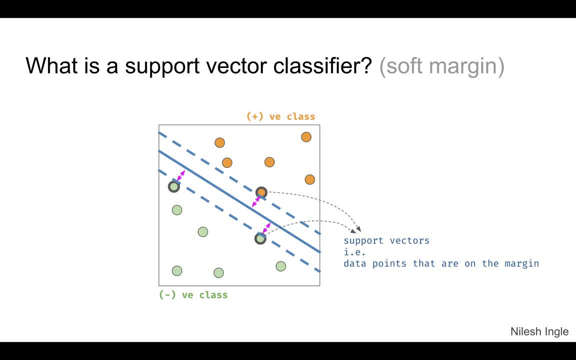 classifier. the idea for the word support is tied to these data points that are associated with this dotted line, so these are called as the support vectors. so these two green dots, and though that orange dot, is the support vector and it's called a support vector because that dotted line is built based on those. 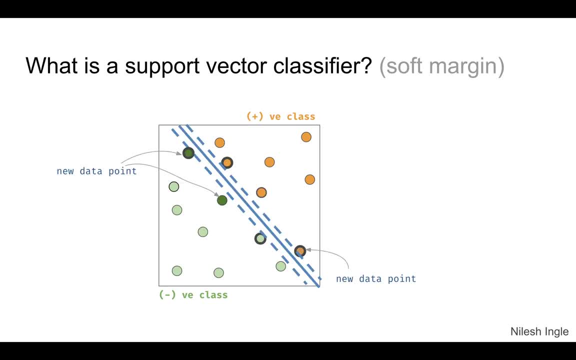 points for each of those classes. now for support. one advantage of support vector classifier is an extra margin. future strength for our classifier muss to be a rest aspect. if so, then we assume that the power vector classifier is the data point. we have already chosen, but gave this an extraеше mama. one aspect was our search, PETER. 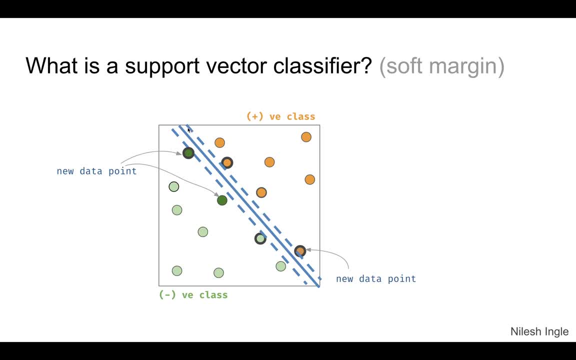 we know that the use case relationship explains that if we just pass a square and ourパ eg profile as 0, alpha makes our black box value and this slice is our number of black boxes with the very relationship with our better and says what if we assume that? 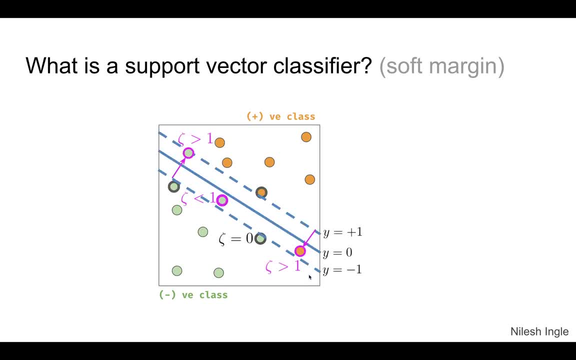 if we choose the filter only and it becomes zero, then this is the maximum margin, with return is 0 to positive ie value equal to 0.5.. and what would the intuition behind that is? we can allow the points to be on the wrong side. 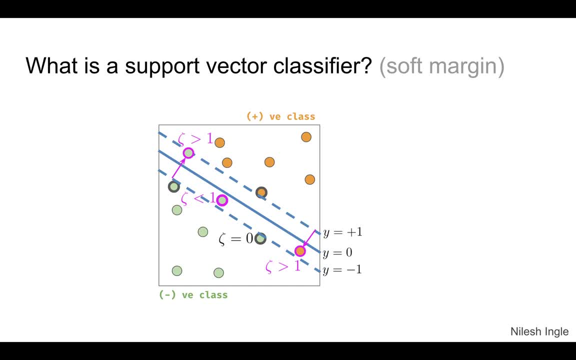 and we can still keep the same decision. so if there is a data point, that's, a new data point comes in, and if it's on the wrong side, that's okay. we do not have to shift our decision boundary substantially. what we can do instead is add a penalty to that particular data point so that it can be, so it will have certain weight. 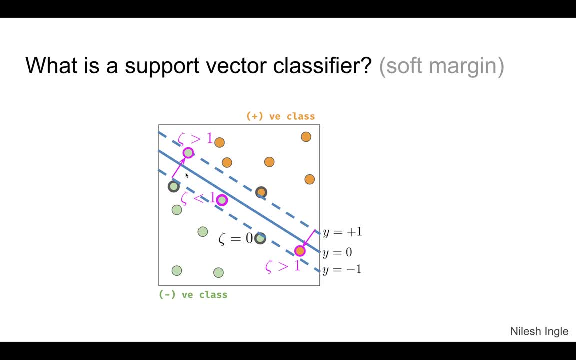 weight of misclassification. so, as we can see in this particular plot, this green dot is on the wrong side so we can add a penalty to that particular data point side. so it's on the orange side and it's away from this decision boundary, and that's also the 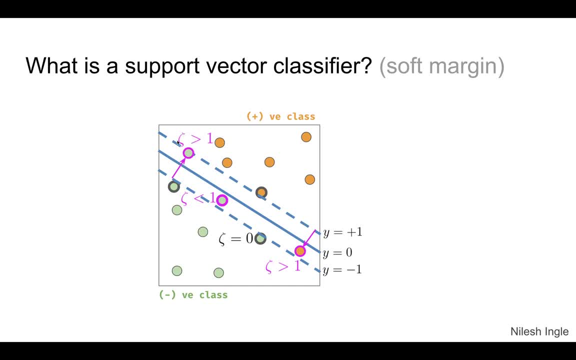 solid line, so the penalty shown here by this greek letter zeta is greater than one. so the farther it is in this direction, the greater would be the value of this particular penalty. and similarly, this orange dot on this side is on the wrong side, and so again the penalty for that would be greater. 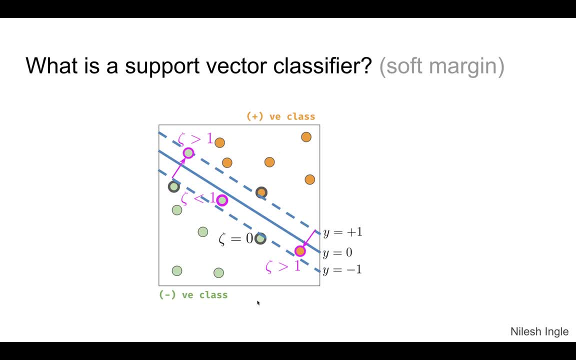 than one and it will continue to increase if it goes farther and farther away from the decision boundary on the wrong side, and here the magenta dot- sorry, the magenta outline. this green dot is on the correct side of the decision boundary. it is classified as a green. 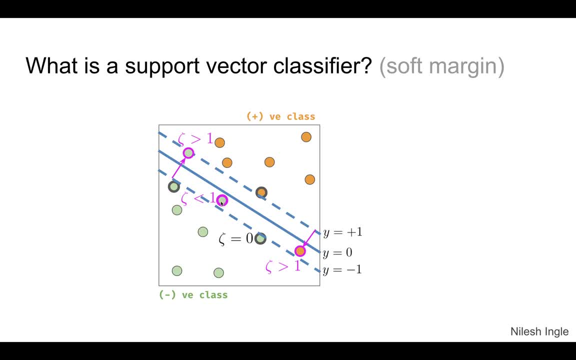 dot. however, it is still within the margin of classification, is inside the dotted line and therefore there would still be a penalty on that, but it would be a smaller penalty because it's correctly classified. it's just that it's within the boundary and in cycle and we can. 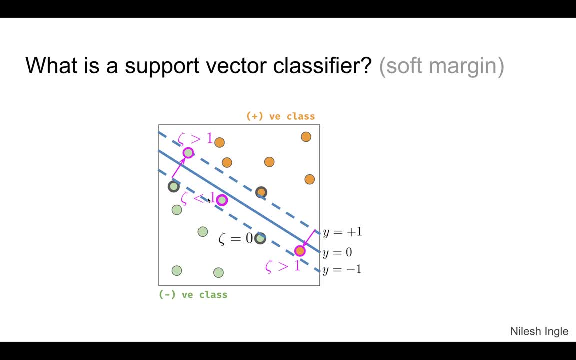 change how flexible we want, how much- uh uh, how much of misclassification we want to allow. we can set that by parameter c, as we'll see, and if the data points are on the right side of the class. so green dots, such as shown here, or the orange dots. 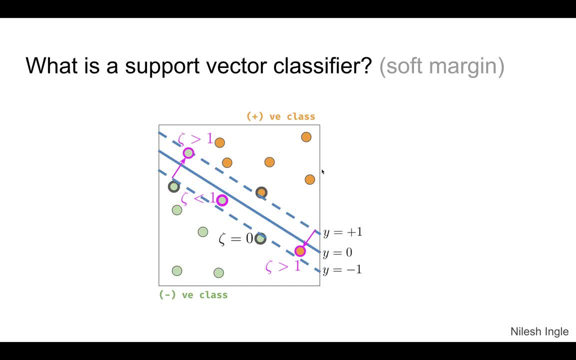 such as shown here, then those would. the zeta value for those would be zero. so there's no penalty for those, because those are correctly classified data points for each of those classes. and here we can see: the value of y is zero for the solid line and then y is equal to plus one for this. 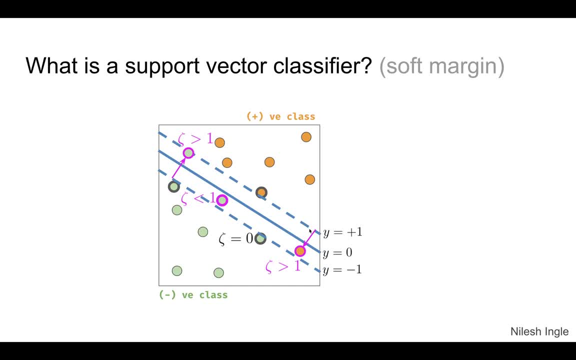 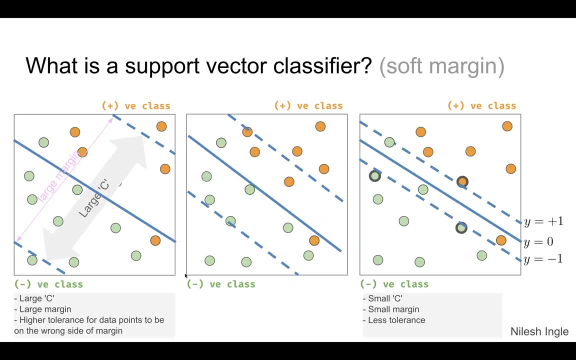 upper margin, margin boundary. and then we have: y is equal to minus one for this lower one. so this we are calling it as a positive class and this we are calling it as a negative class. now, as mentioned earlier, we can tune how much of the misclassification we want to allow. 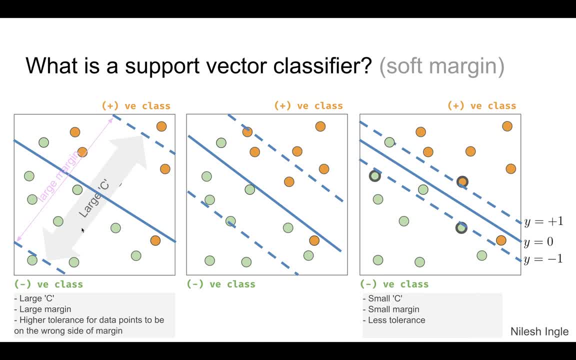 so how much are data points we think would be okay if they are on the wrong side and that can be set by a parameter, c. so if the value of c is large, then we get a larger margin. so the distance between these two dotted lines would be much larger, and so there will be more room for the data points to 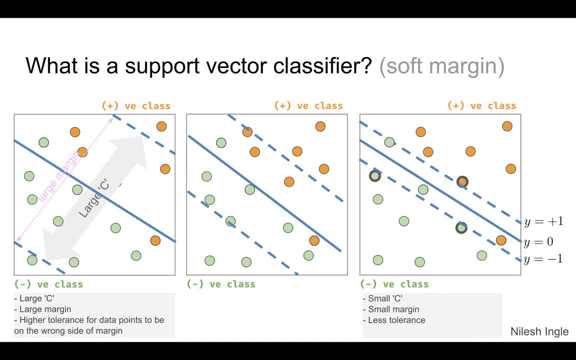 stay on either side, but still the value of z is equal to minus one for this lower one, so zeta would be much lesser. so we are kind of allowing the data points to be where they want and still not care about adding too much penalty on them. but as we start to reduce the value of c, 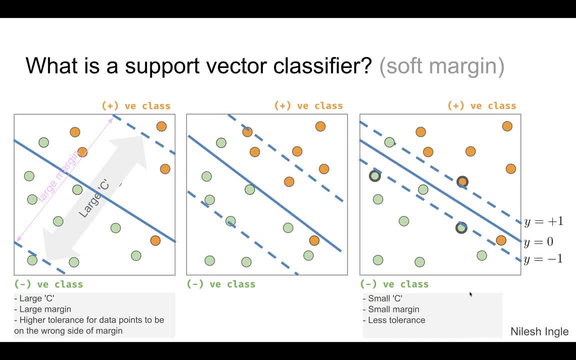 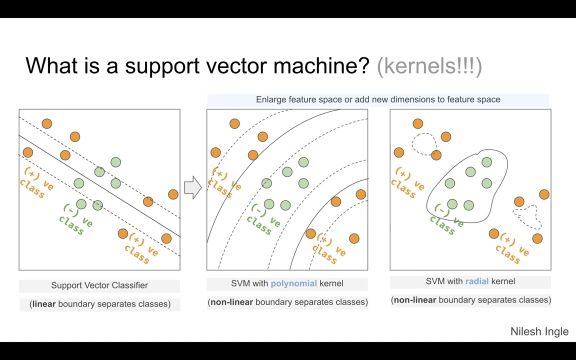 we see that this margin becomes narrower and then, with a small margin, there is indeed a lesser tolerance for misclassification, or lesser tolerance that the data points would be on the wrong side of the margin. now what support mector machine is then? it builds upon all those ideas and introduces or adds a new. 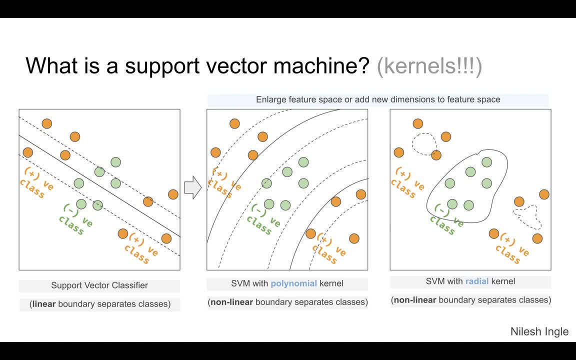 capability of kernels. as we have seen in the previous video on kernels, the central idea with using kernels is that let's say you have a data set of kernels and you have a data set of kernels and you have a data set of kernels and that's in two dimensions that cannot be separated in linearly or that cannot be separated, then what? 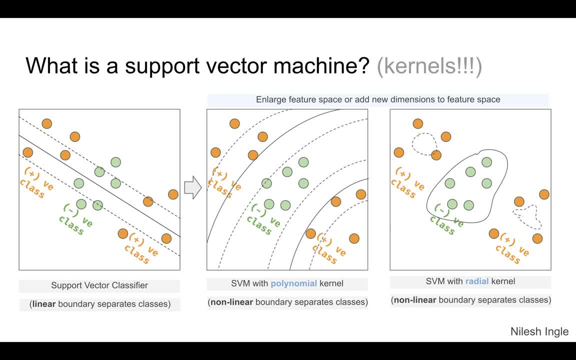 you do is you take, you add dimension to that data set, project it in a, let's say, two-dimensional data set into three-dimensional data set- and they're using kernels- and then you'll see that the points magically separate into- maybe some points stay higher up and some points. 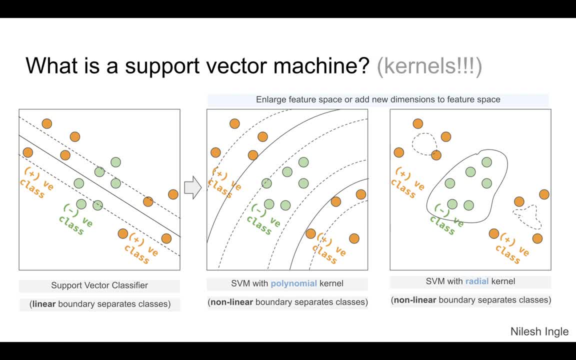 lower down, so then the higher class and lower class could be easily separated in that dimension. so that's the general idea. if you're still not sure about how kernels work, i suggest checking out the video on kernels. i think it was about four or five videos back. so here what we have is: 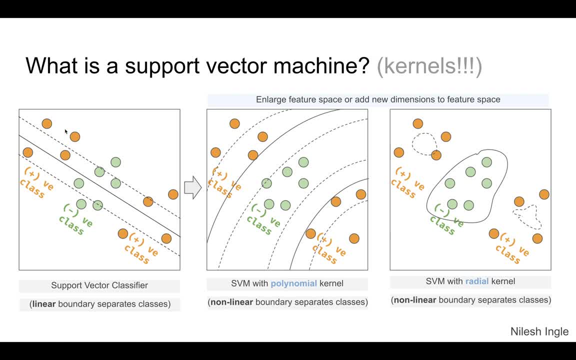 on the left hand side we have a data set. we still have two classes: the orange dots and the green dots. however, in this case, the orange, the green dots are with kind of sandwiched between the orange dots on either side, and so if we use a straight linear classifier, then it's not able to separate this. if we draw a straight line. this 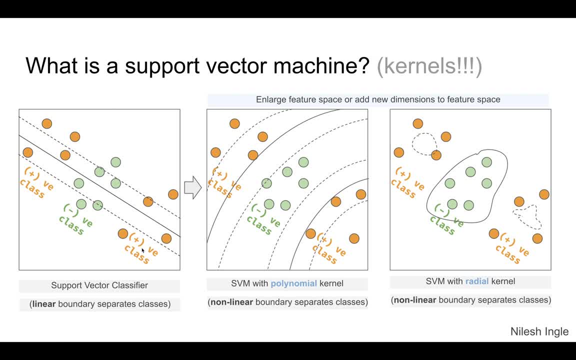 we could draw a line like this or like this, or either way. we cannot clearly separate the green and you the orange dots. so the solution to solving this type of classification problem is using a line that is not straight, so using a non-linear line, and in the figure in the middle you can. 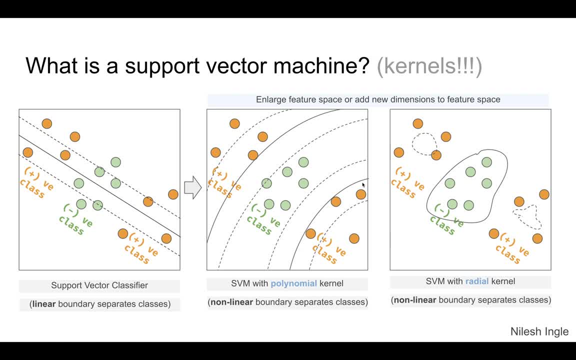 see that if we use a polynomial kernel, then we have this line, which is non-linear, it has curved line and we could separate these orange dots and the green dots, as shown here. another variation or another type of kernel which is also commonly used is the radial basis. 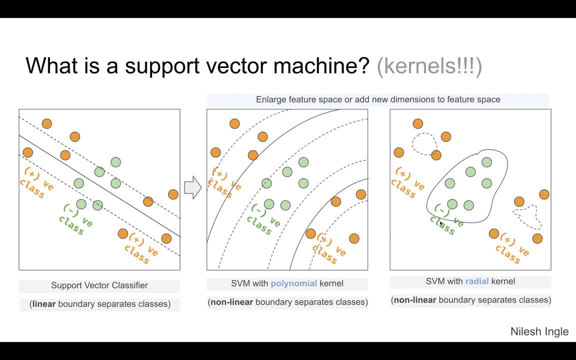 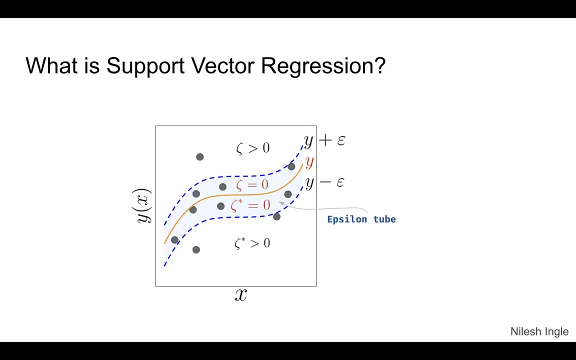 function based the radial kernel, and what that does is it would clearly separate these green data points from the orange data points, as shown here. you, and that's possible because they would use the non-linear boundary to separate those two classes. and while so far we have talked about support vector classifiers, now let's talk about support. 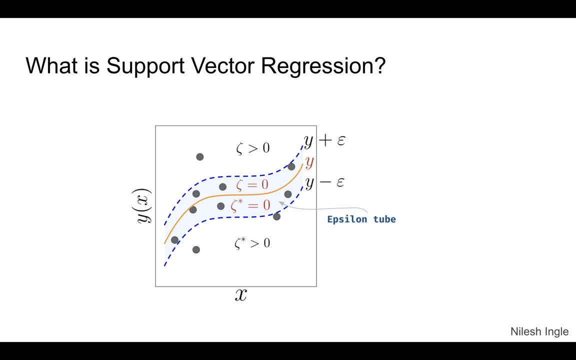 vector regression on this slide. so we have talked about this briefly in the previous videos. so the idea is that we are looking at the epsilon. so the idea is that we are looking at the epsilon. so the idea is that we are looking at the epsilon tube which is shown here in the blue. 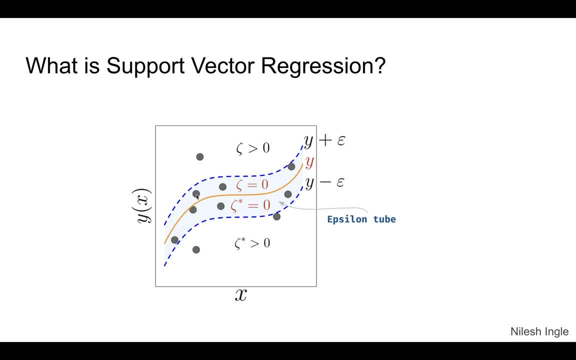 tube which is shown here in the blue tube, which is shown here in the blue shaded region. so if we have data points shaded region, so if we have data points shaded region, so if we have data points which are which are, which are black dots that are shown here, then the 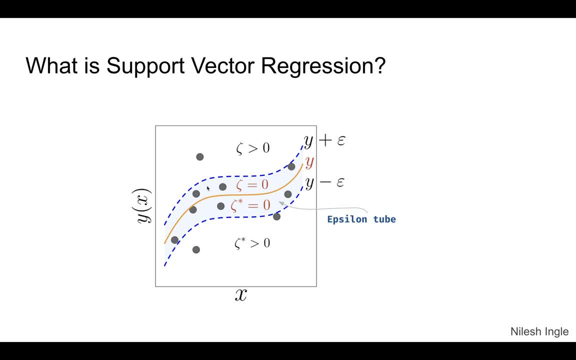 black dots that are shown here, then the black dots that are shown here, then the main idea is that we want. main idea is that we want. main idea is that we want the, the, the data points to be within this epsilon, data points to be within this epsilon. 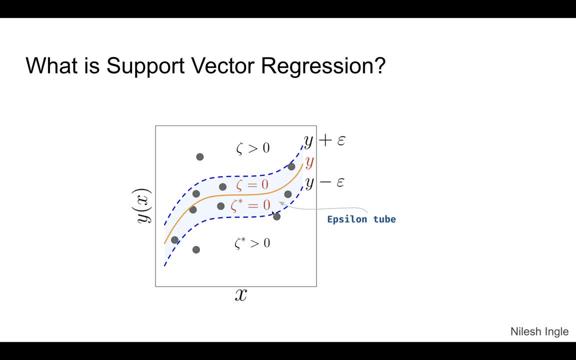 data points to be within this epsilon tube. if they are within this epsilon tube tube, if they are within this epsilon tube tube, if they are within this epsilon tube, then there is no penalty associated with then there is no penalty associated with, then there is no penalty associated with those data points. however, if the data 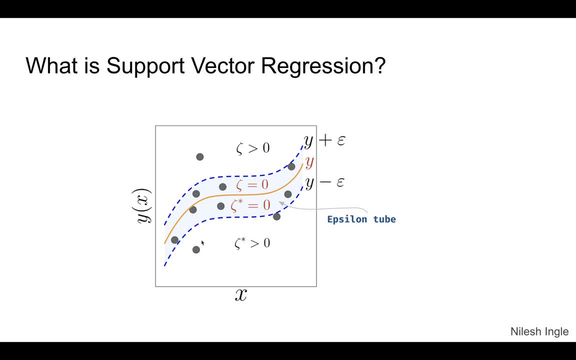 those data points. however, if the data, those data points, however, if the data points lie outside these data, these, this points lie outside these, this points lie outside these. this epsilon tube, then there is a penalty. epsilon tube, then there is a penalty. epsilon tube, then there is a penalty associated with those data points. so as 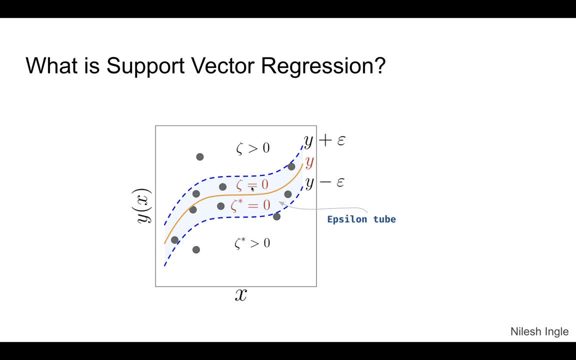 associated with those data points. so as associated with those data points. so as you can see the, you can see the. you can see the letters zeta here c is equal to zero if letters zeta here c is equal to zero. if letters zeta here c is equal to zero. if the data points are above: 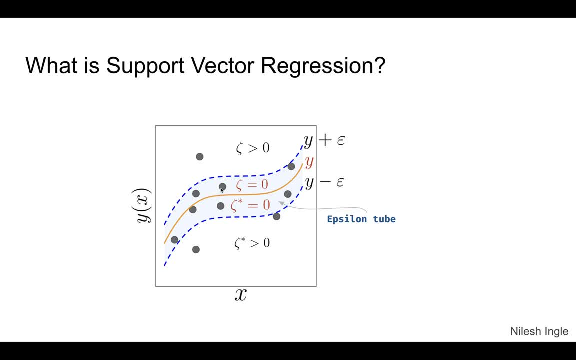 the data points are above. the data points are above this orange line in the middle, this orange line in the middle, this orange line in the middle and still in the, and still in the and still in the epsilon tube. however, if the data point and still in the epsilon tube, however, if the data point is outside, such as zone, 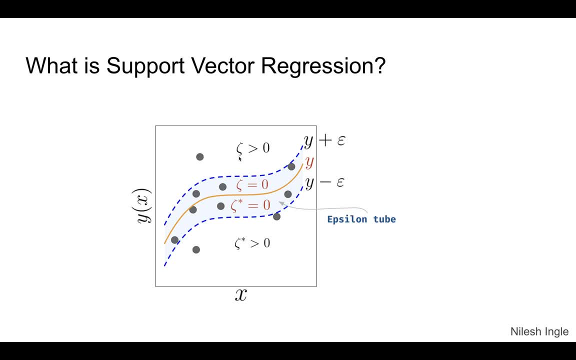 is outside, such as zone is outside, such as zone here. then for that data point, there will here. then for that data point, there will here. then for that data point, there will be a penalty and the be a penalty and the be a penalty and the zeta value would be greater than zero. 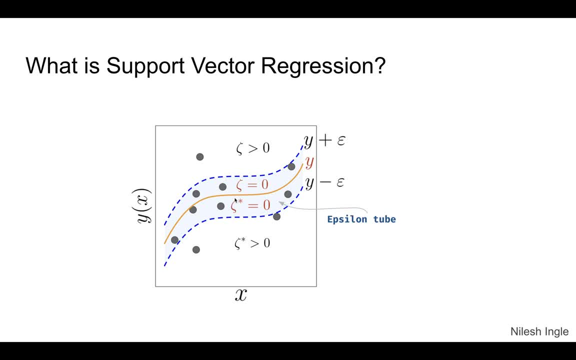 zeta value would be greater than zero. zeta value would be greater than zero. similarly, if the data points are similarly, if the data points are similarly, if the data points are below the this orange line, below the this orange line, below the this orange line, then it's uh marked by zeta star still. 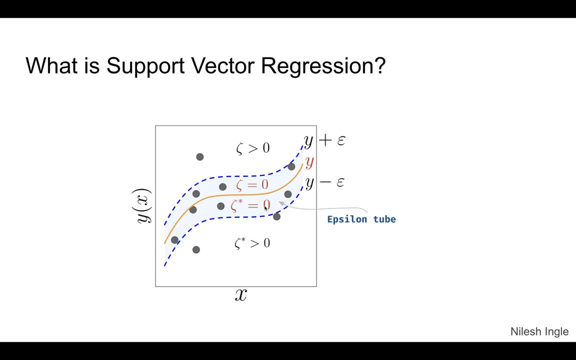 then it's uh marked by zeta star. still then it's uh marked by zeta star. still equal to zero, equal to zero, equal to zero. because they are within the epsilon tube, because they are within the epsilon tube, because they are within the epsilon tube. that is this blue shaded area, and 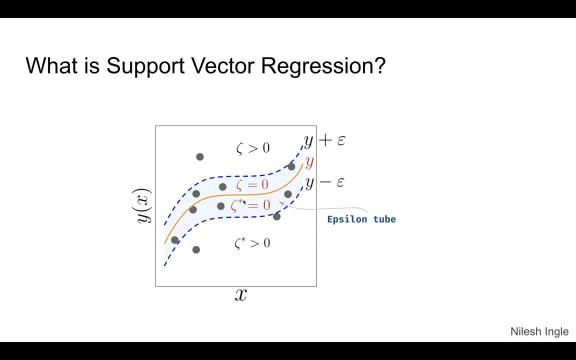 that is this blue shaded area, and that is this blue shaded area. and, however, if they are outside that, however, if they are outside that, however, if they are outside that farther away from that, then, as you go farther away from that, then, as you go farther away from that, then, as you go farther away, the value of the zeta star. 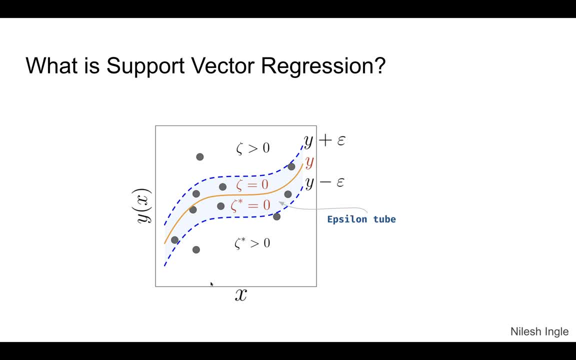 farther away, the value of the zeta star, farther away, the value of the zeta star would, would, would, uh would increase. so you're adding more uh would increase. so you're adding more uh would increase. so you're adding more and more penalty for and more penalty for. 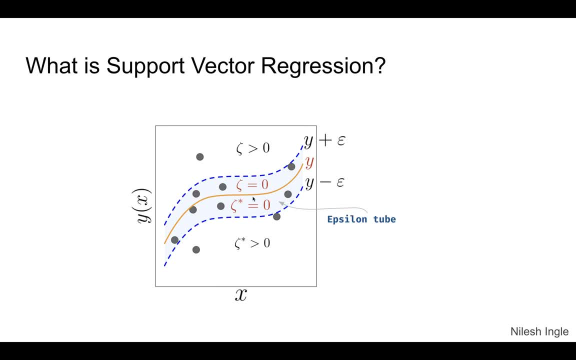 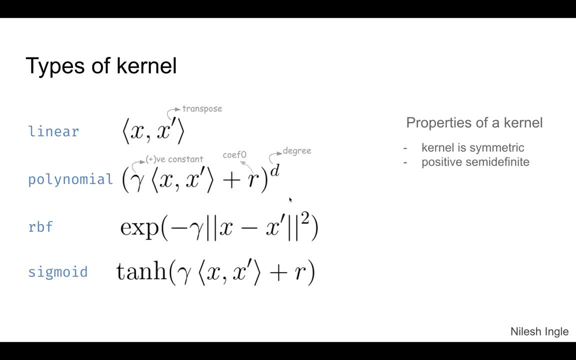 and more penalty for that particular data point which is away, that particular data point which is away, that particular data point which is away from the existing data points, within from the existing data points, within from the existing data points within this epsilon tube, this epsilon tube, this epsilon tube, now the types of kernels that are used. 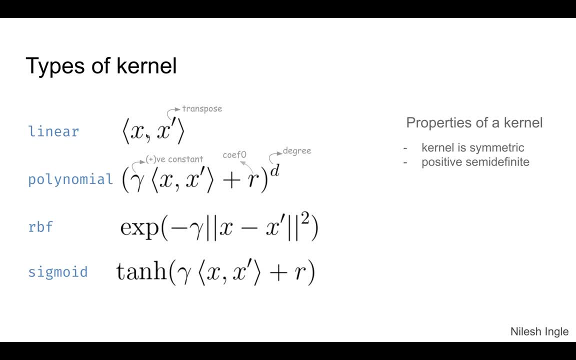 now the types of kernels that are used now. the types of kernels that are used in the scikit-learn for in the scikit-learn for in the scikit-learn for support vector machines are shown here. support vector machines are shown here. support vector machines are shown here. we have a linear kernel. we have 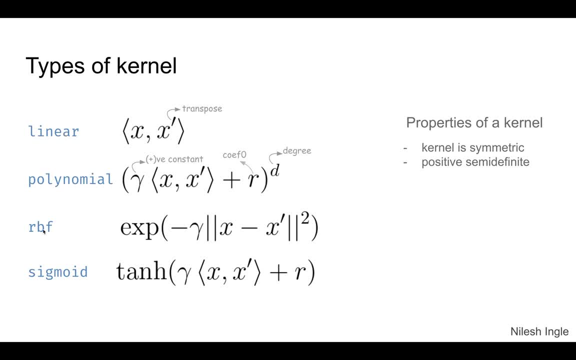 we have a linear kernel. we have we have a linear kernel. we have polynomial kernel. we have rbf radial polynomial kernel. we have rbf radial polynomial kernel. we have rbf radial basis function. we have sigmoid basis function. we have sigmoid basis function. we have sigmoid kernel. and these are the equations that 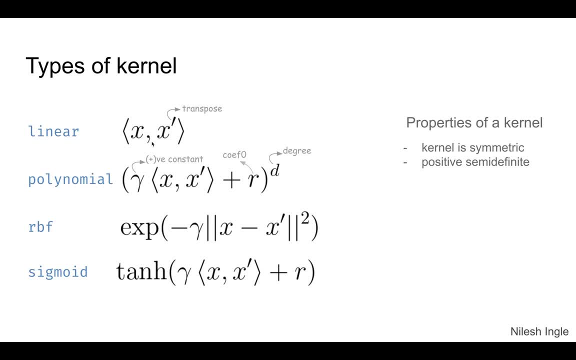 kernel and these are the equations that kernel and these are the equations that are shown, are shown, are shown for all these types of kernels, and this for all these types of kernels and this for all these types of kernels, and this angle bracket just shows that it's a 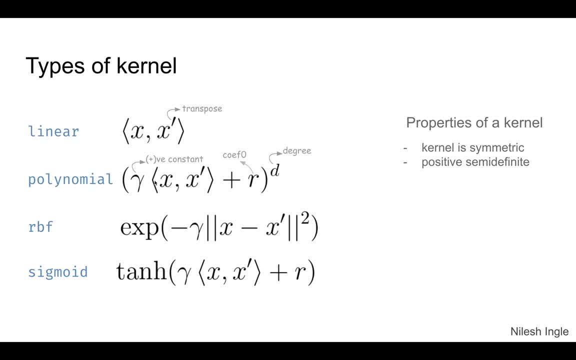 angle bracket just shows that it's a angle bracket just shows that it's a dot product between x and x transpose. dot product between x and x transpose. dot product between x and x transpose. and this is fun for polynomial we have. and this is fun for polynomial we have. 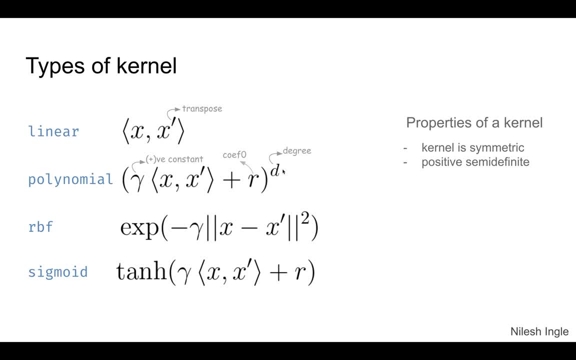 and this is fun for polynomial. we have this degree that we can use, so you can this degree that we can use, so you can this degree that we can use, so you can use a. use a. use a. nth second order, third order fourth: nth second order, third order, fourth: 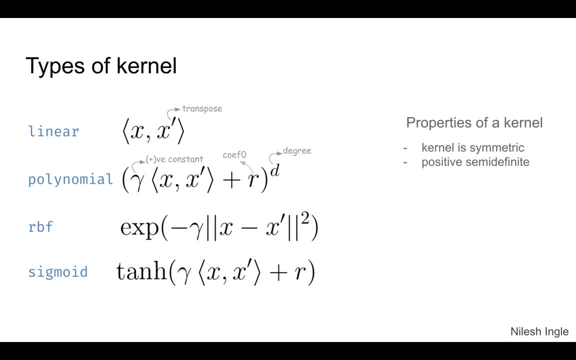 nth. second order. third order, fourth order: polynomial based on order: polynomial based on order. polynomial based on how: how complicated the data is, how. how complicated the data is how. how complicated the data is and how and how and how. how much of wiggle room you need to. 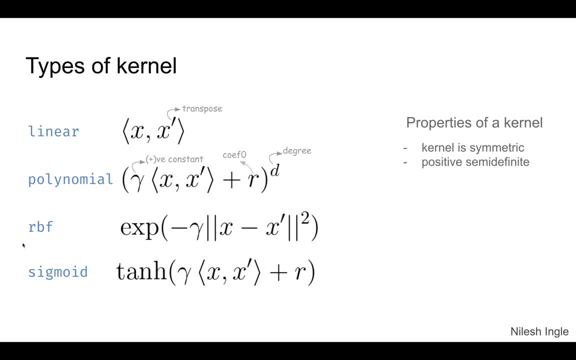 how much of wiggle room you need to, how much of wiggle room you need to separate. classify those data points separate. classify those data points separate. classify those data points. and then we have the rbf that we saw. and then we have the rbf that we saw. 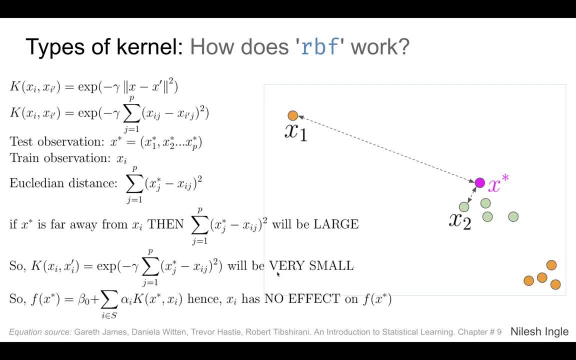 and then we have the rbf- that we saw- and we have the sigmoid, and we have the sigmoid, and we have the sigmoid. now, how does the rbf kernel work? so now, how does the rbf kernel work? so now, how does the rbf kernel work? so let's start from the 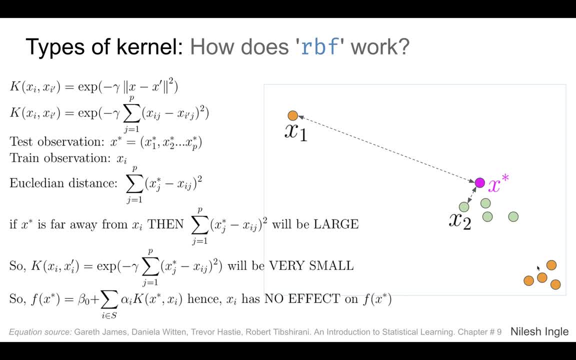 let's start from the. let's start from the figure on the right hand side here. if we figure on the right hand side here, if we figure on the right hand side here, if we have these data points, have these data points, have these data points that are the orange, orange data points. 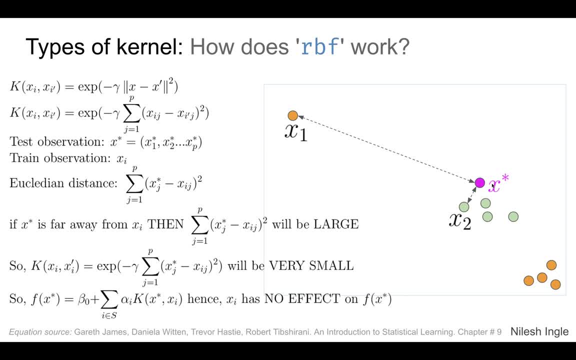 that are the orange orange data points. that are the orange orange data points. right, one is right there. there are a right. one is right there. there are a right. one is right there. there are a couple here, couple here, couple here, and we have the green dots that are. 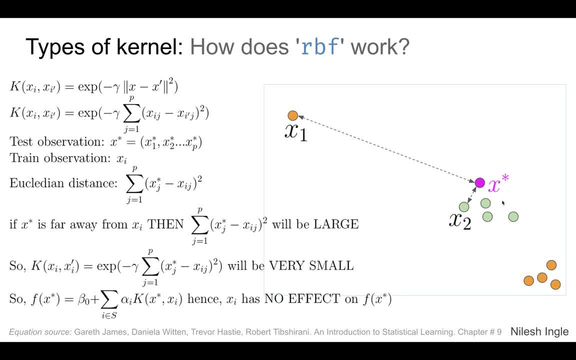 and we have the green dots that are, and we have the green dots that are sandwiched within those orange, sandwiched within those orange, sandwiched within those orange data points now if a new data point? data points now if a new data point. data points now if a new data point comes in. 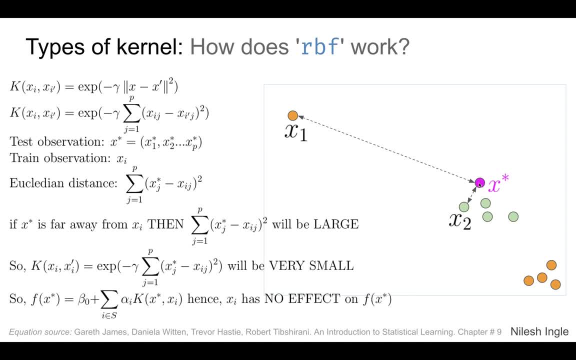 comes in, comes in. let's say this magenta data point and let's say this magenta data point and let's say this magenta data point and we need to classify that. so how would we need to classify that? so how would we need to classify that? so how would rbf? 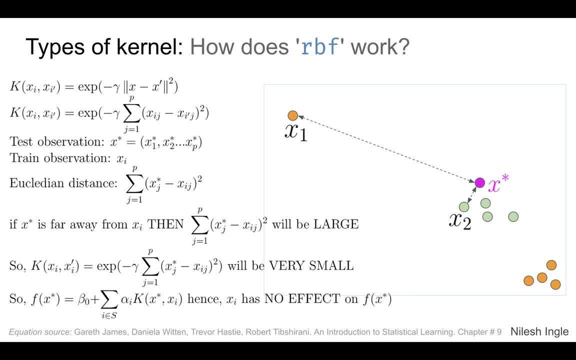 rbf, rbf classify how. how would rbf classify how? how would rbf classify how? how would rbf work? so if we look at the radial basis work, so if we look at the radial basis work, so if we look at the radial basis function, function. 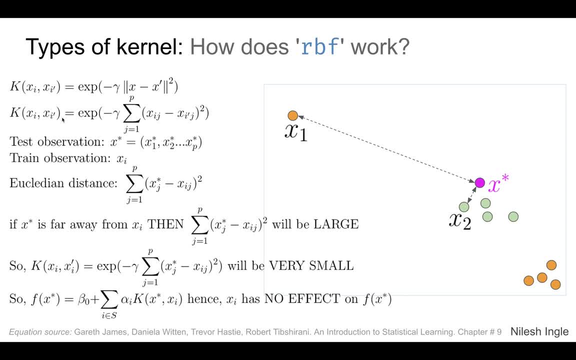 function. that's shown here in the top. that's shown here in the top. that's shown here in the top. if a new data point comes in, which, let's. if a new data point comes in which, let's. if a new data point comes in which, let's say it is. 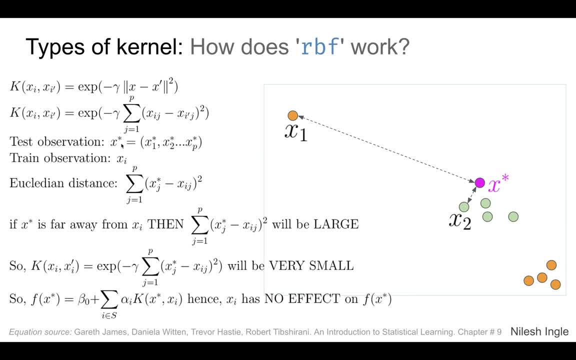 say it is, say it is x star, then based on that, we can x star. then based on that, we can x star. then, based on that, we can see, we can think of the test observation. see, we can think of the test observation. see, we can think of the test observation. as x star is equal to: 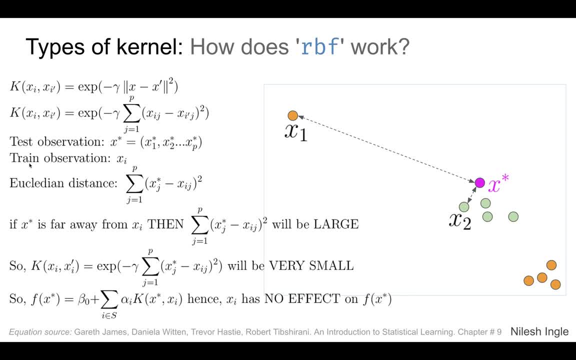 as x star is equal to. as x star is equal to x1 star, x2 star, xp star, and then the x1 star, x2 star, xp star, and then the x1 star, x2 star, xp star, and then the trend observation would be equal to xi. 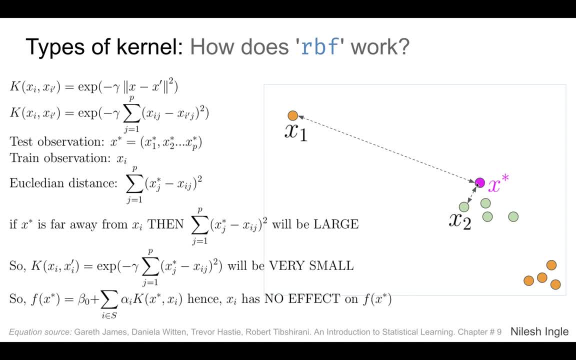 trend observation would be equal to xi. trend observation would be equal to xi. and now if we calculate the euclidean, and now if we calculate the euclidean, and now if we calculate the euclidean distance between this data point and distance between this data point, and distance between this data point and this data point, we can calculate it by: 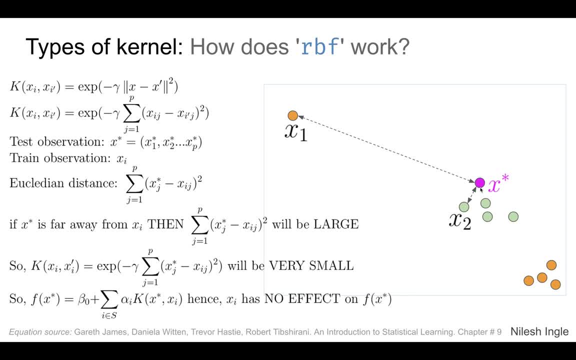 this data point. we can calculate it by this data point, we can calculate it by this formula. and if this euclidean this formula, and if this euclidean this formula, and if this euclidean distance, distance- distance is very large, for example in this case, is very large, for example, in this case: 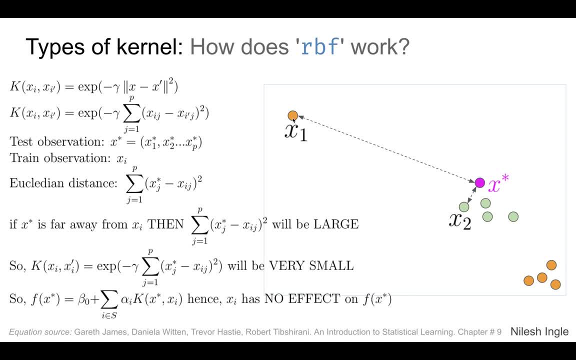 is very large. for example, in this case, the distance between the magenta dot, the distance between the magenta dot, the distance between the magenta dot and the x1 orange dot would be much and the x1 orange dot would be much and the x1 orange dot would be much larger if, if you have a large number, 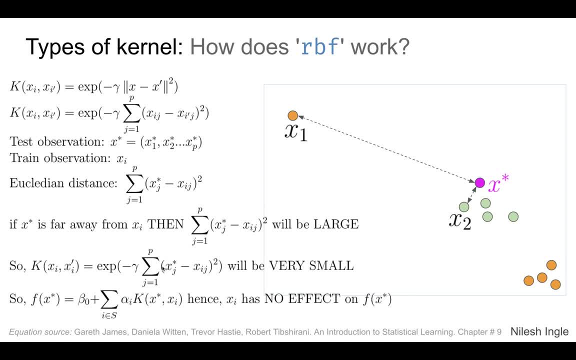 larger if, if you have a large number, larger, if, if you have a large number, then when you, then when you, then when you put that number in this expression, when put that number in this expression, when put that number in this expression, when you try to get an exponential for that. 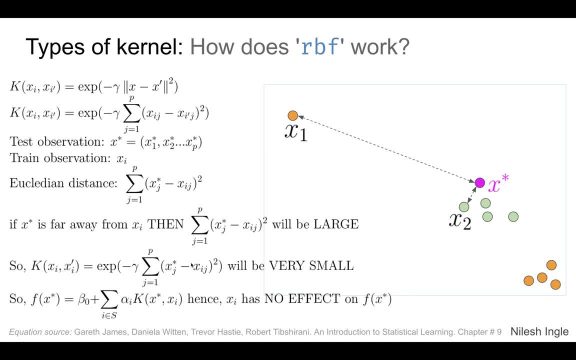 you try to get an exponential for that. you try to get an exponential for that. when calculating the, when calculating the, when calculating the kernel, then that value would be very kernel, then that value would be very kernel, then that value would be very small and small and small and the value value for that data point. 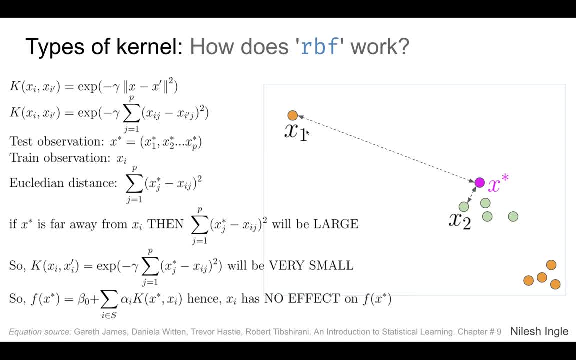 the value value for that data point. the value value for that data point would be very small in the kernel, would be very small in the kernel, would be very small in the kernel, and so and so and so, essentially this particular data point, essentially this particular data point. 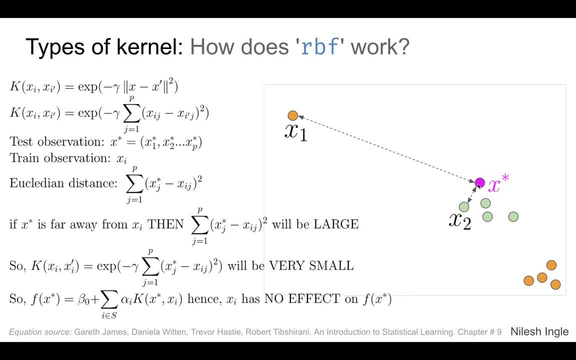 essentially, this particular data point would have no effect in, would have no effect in, would have no effect in flipping the sign of this. flipping the sign of this, flipping the sign of this decision function to classify this as a decision function. to classify this as a decision function. to classify this as a positive or negative class. 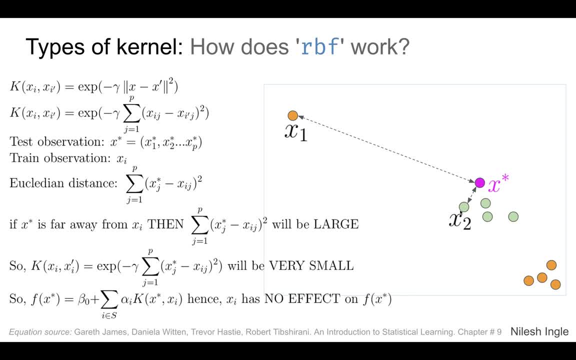 positive or negative class, positive or negative class, so, so, so the most effect would be from the closest. the most effect would be from the closest, the most effect would be from the closest point. that is here point, that is here point. that is here to, to, to. so this point would dominate what the 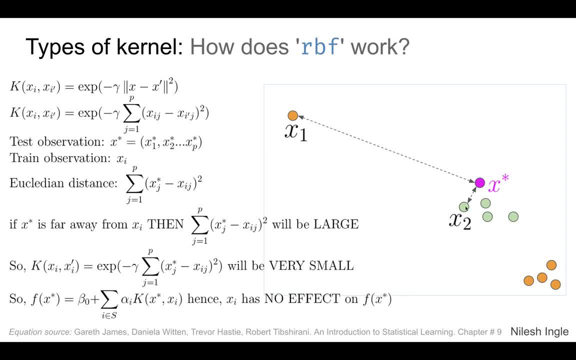 so this point would dominate what. the. so this point would dominate what. the sign of the sign of the sign of the decision, sign of the output of the decision, sign of the output of the decision, sign of the decision function would be. would it be positive? decision function would be. would it be positive? 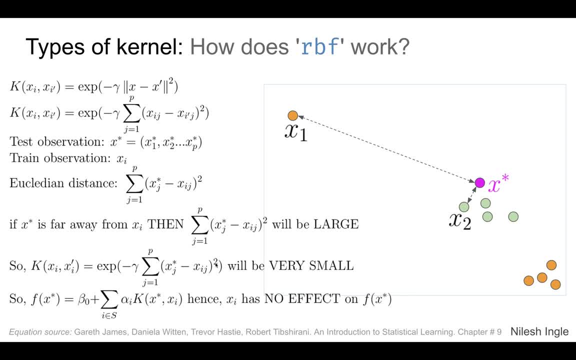 decision function would be: would it be positive or negative, or negative or negative? to assign that data point to either a. to assign that data point to either a. to assign that data point to either a positive or negative class, positive or negative class, positive or negative class. so that that's kind of the general. 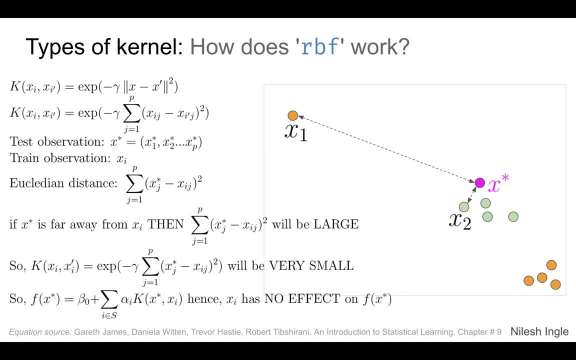 so that that's kind of the general. so that that's kind of the general intuition of how the rbf work, intuition of how the rbf work. intuition of how the rbf work: uh, rbf kernel would work. uh, rbf kernel would work. uh, rbf kernel would work. and i've put a reference below, if you. 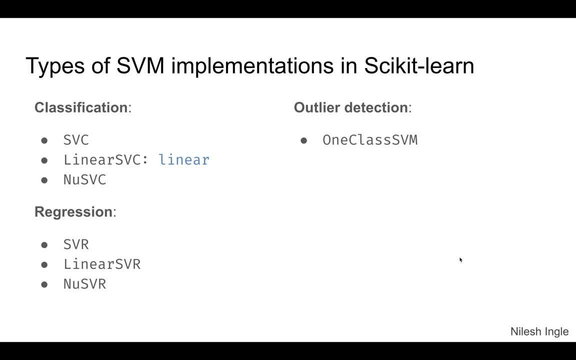 and i've put a reference below. if you and i've put a reference below, if you want to read further in on this topic, want to read further in on this topic. want to read further in on this topic. now in scikit-learn, there are different. 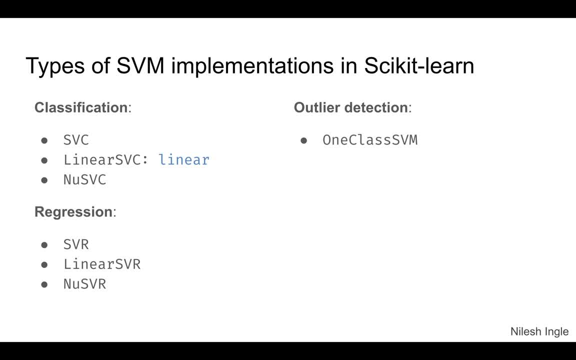 now in scikit-learn there are different. now in scikit-learn there are different implementations: uh for svm. we have implementations uh for svm. we have implementations uh for svm. we have for classification and regression, we for classification and regression, we for classification and regression. we have svc, linear svc, new svc. 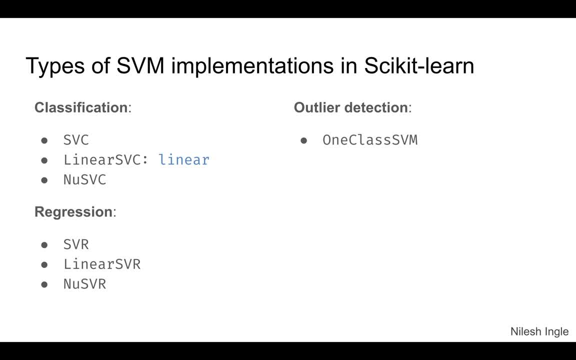 have svc, linear svc, new svc, have svc, linear svc, new svc, and then and then and then for regression, we have svr for regression, we have svr for regression. we have svr, linear svr and new svr, linear svr and new svr, linear svr and new svr. now the new svc and new svr, it's 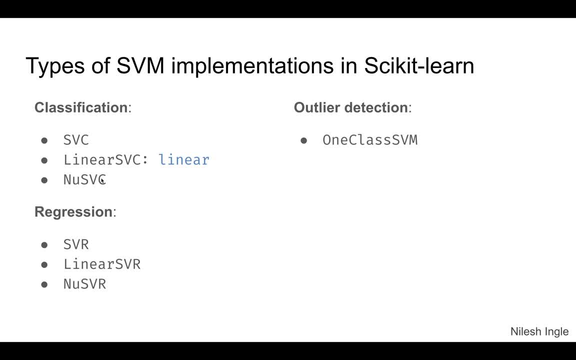 now the new svc and new svr. it's now the new svc and new svr. it's uh, uh, uh. a version where there is a parameter, a version where there is a parameter, a version where there is a parameter. new instead of c, new instead of c. 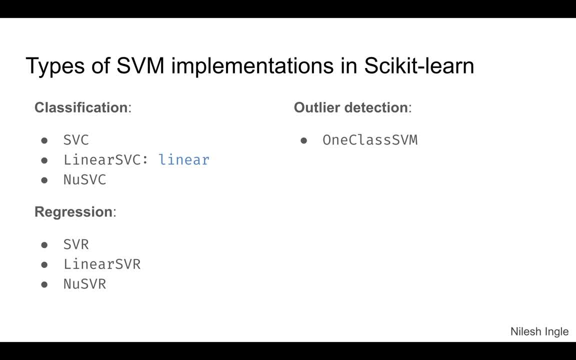 new instead of c, and that controls the regularization, and that controls the regularization and that controls the regularization. that's within, that's within, that's within, within the function, so within the function, so within the function. so that's the change, and that's the change, and that's the change. and with one class, svm. this is 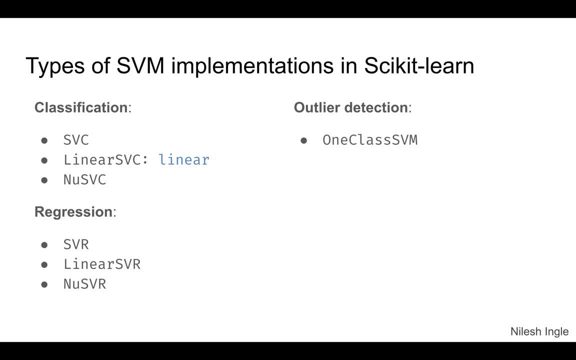 with one class svm. this is with one class svm. this is uh it generally, uh it generally, uh it generally are used to find outliers and are used to find outliers and are used to find outliers, and so that's so, that's so, that's a separate, a separate. 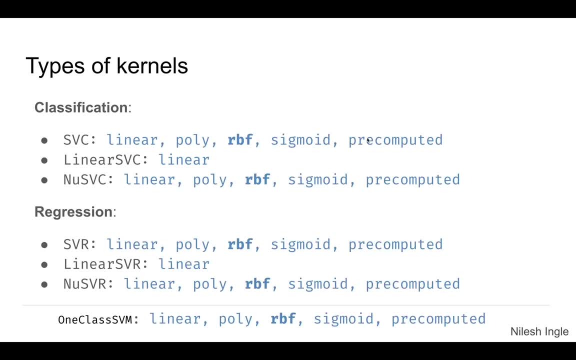 a separate method that we have available method that we have available method that we have available the types of kernels that we can use, the types of kernels that we can use, the types of kernels that we can use with each of these methods. with each of these methods. 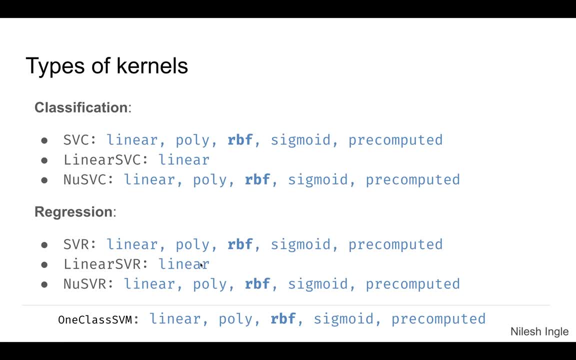 with each of these methods. for linear, we just have the linear. for linear, we just have the linear for linear. we just have the linear method, as we would expect, however, for method as we would expect, however, for method as we would expect, however, for all other methods we can use. 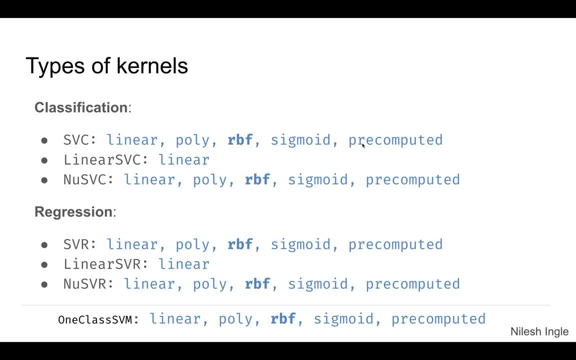 all other methods. we can use all other methods. we can use all the four types of kernels that we all the four types of kernels that we all, the four types of kernels that we saw earlier. in addition, we can use a saw earlier. in addition, we can use a. 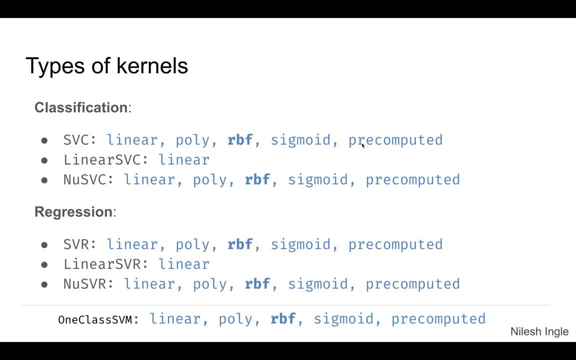 saw earlier. in addition, we can use a pre-computed, pre-computed, pre-computed custom funnel, custom kernel. so if you custom funnel, custom kernel, so if you custom funnel, custom kernel, so if you have a specific, have a specific, have a specific kernel, kernel, kernel. so let's say you have a data set that 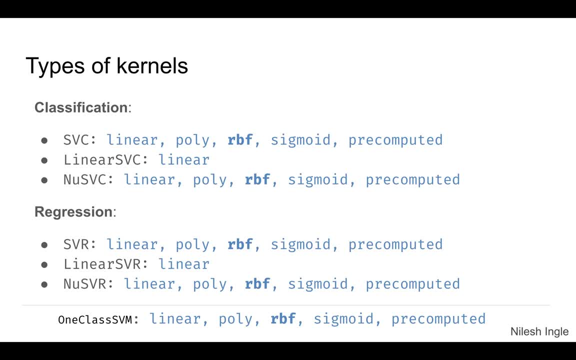 so let's say you have a data set that. so let's say you have a data set that needs to, needs to, needs to, that can be, that can be, that can be easily classified, easily classified, easily, classified only and only if only and only if only and only if it can be. 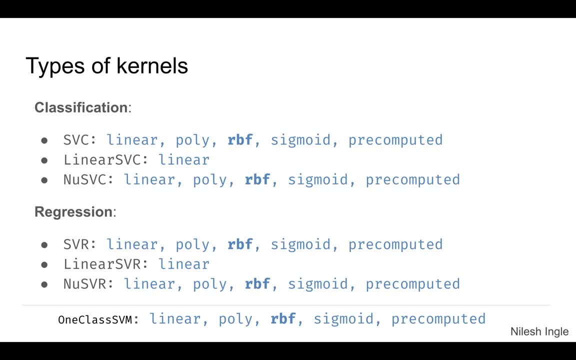 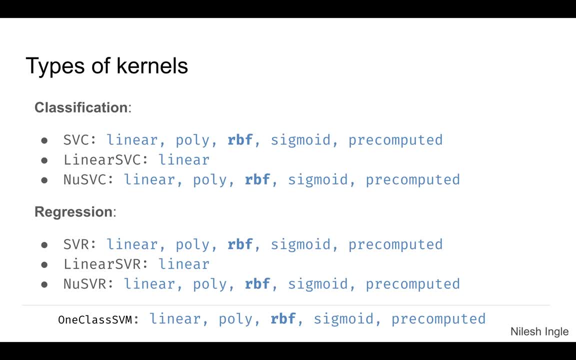 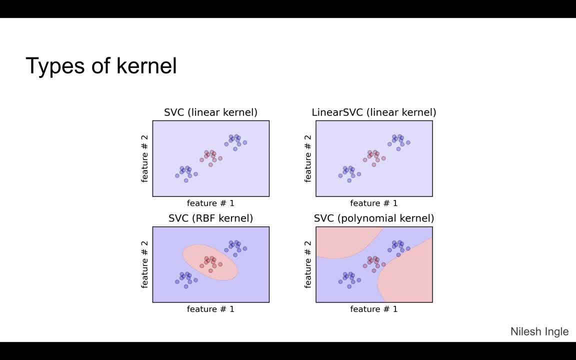 listed here. listed here, and this is the actual run of and this is the actual run of and this is the actual run of these different kernels and different these different kernels and different these different kernels and different methods that i wanted to share, methods that i wanted to share. 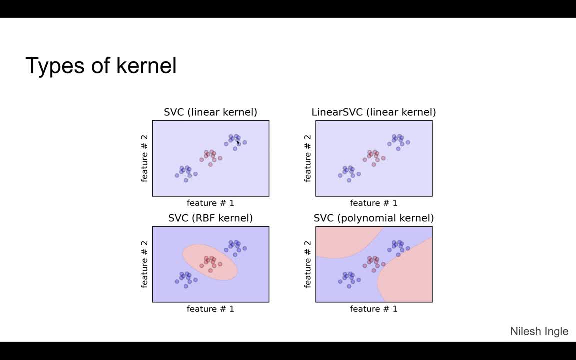 methods that i wanted to share. and here we have these blue data points, and here we have these blue data points, and here we have these blue data points and within and within and within, those is sandwiched, this, those is sandwiched, this, those is sandwiched this- red data points. and if we try to 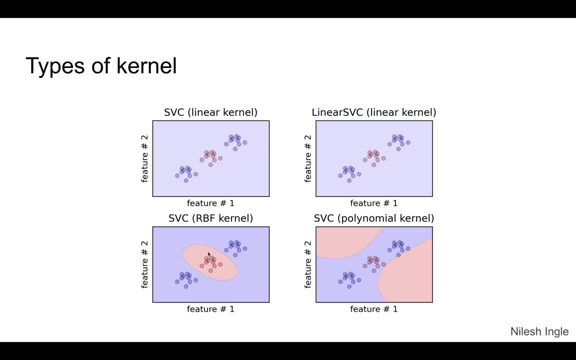 red data points and if we try to red data points and if we try to separate them by either of these, separate them by either of these, separate them by either of these methods, methods, methods. uh, this rbf method, uh, this rbf method. uh, this rbf method was very good at. 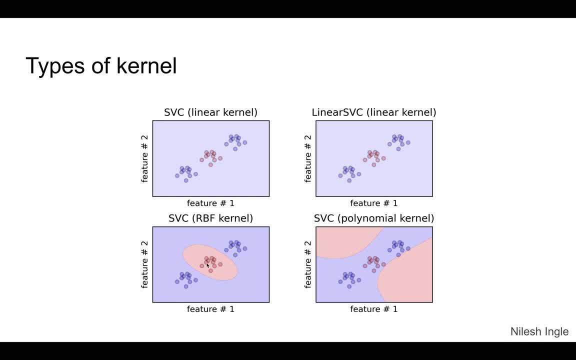 was very good at, was very good at cleanly isolating those, cleanly isolating those, cleanly isolating those data points in middle data points, in middle data points, in middle polynomial. this was, i think, around nine polynomial. this was, i think, around nine polynomial. this was, i think, around nine degree, and still it was. 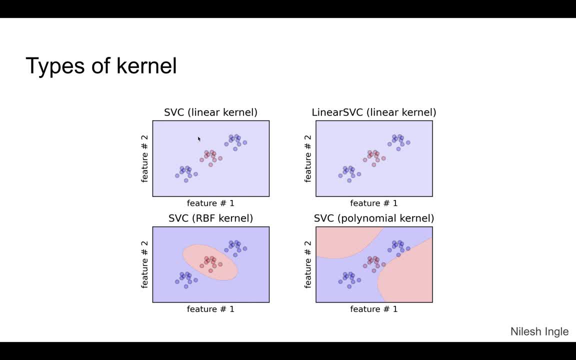 degree and still it was degree and still it was struggling to get those out, struggling to get those out, struggling to get those out. linear models were linear models were linear models were definitely this problem, definitely this problem, definitely this problem. i was out of reach and they are not. 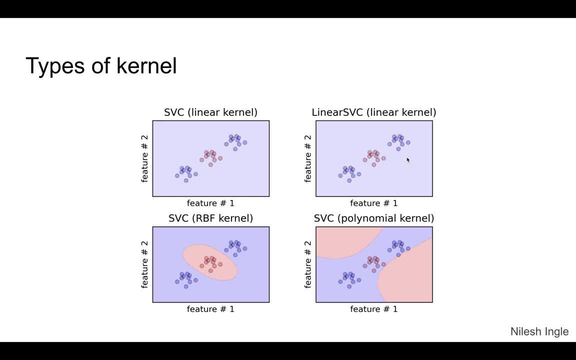 i was out of reach and they are not. i was out of reach and they are not able to classify those two different. able to classify those two different, able to classify those two different classes, classes, classes, and similarly, if we increase the and similarly, if we increase the, 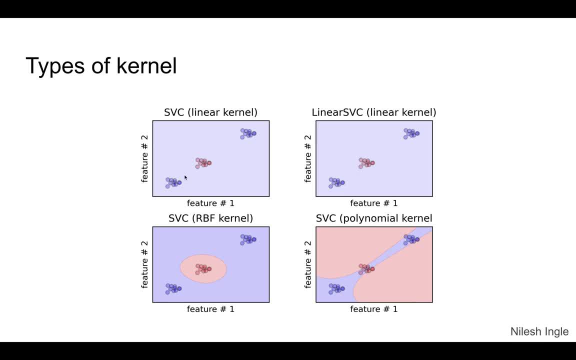 and similarly, if we increase the distance between distance, between distance between these classes, i thought maybe that these classes, i thought maybe that these classes, i thought maybe that will give, will give, will give some different, some different, some different effect and the radial basis again, effect and the radial basis again. 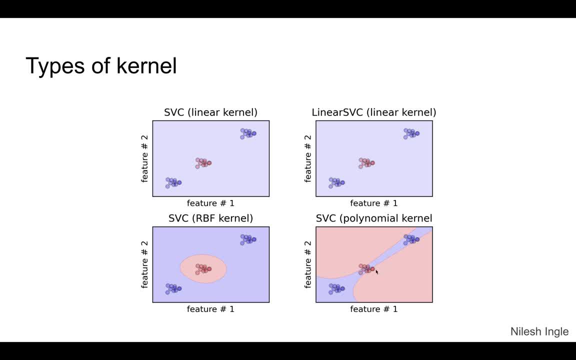 effect and the radial basis again was able to classify, was able to classify, was able to classify the polynomial kernel, the polynomial kernel, the polynomial kernel. now, now, now, maybe it was getting closer to, maybe it was getting closer to, maybe it was getting closer to classifying. it did get some of the 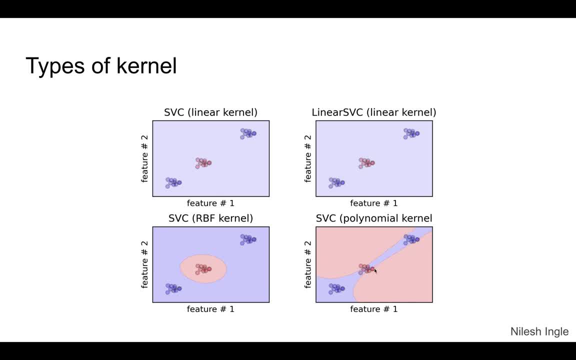 classifying. it did get some of the classifying. it did get some of the points as compared to here, but then still points as compared to here, but then still points as compared to here, but then still, in this particular scenario it was difficult to separate them using 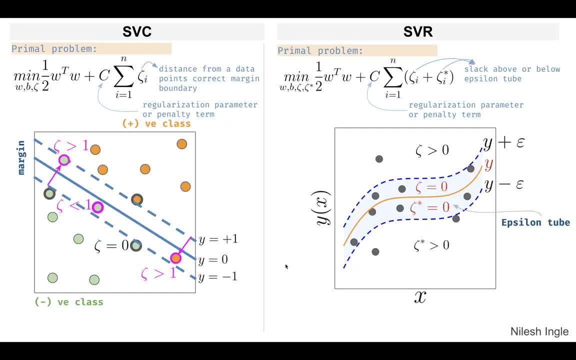 it was difficult to separate them using. it was difficult to separate them using polynomial as well. now the support vector classifier and now the support vector classifier, and now the support vector classifier and support vector regression. so if we support vector regression, so if we support vector regression, so if we want to get some mathematical intuition, 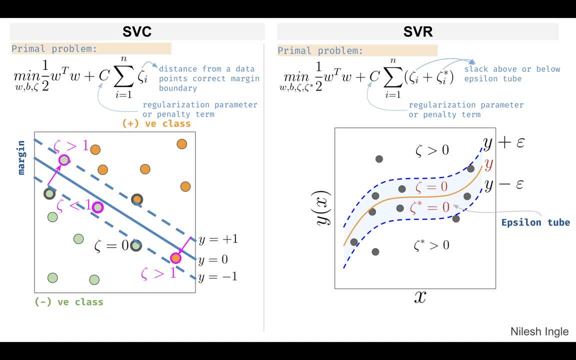 want to get some mathematical intuition, want to get some mathematical intuition. this is not a derivation. this is not a derivation. this is not a derivation. i'm just going to walk through. i'm just going to walk through, i'm just going to walk through the equations that 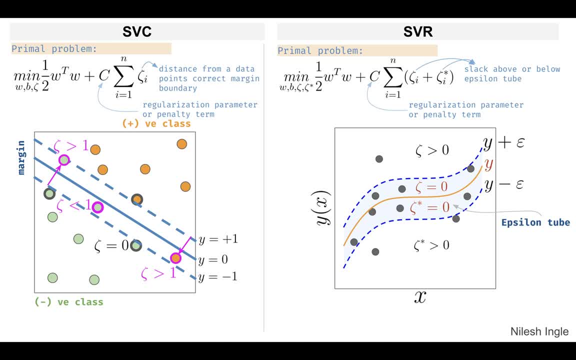 the equations, that the equations that are listed in the docs and try to try to talk about, what those equations try to talk about, what those equations try to talk about, what those equations could be telling, could be telling, could be telling: and here the and here the and here the for each of those two. 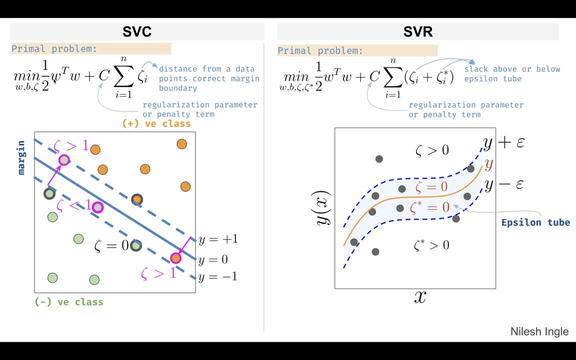 for each of those two, for each of those two types. we have this minimization problem types. we have this minimization problem types. we have this minimization problem where we have w transpose w, where we have w transpose w, where we have w transpose w that we have seen before and 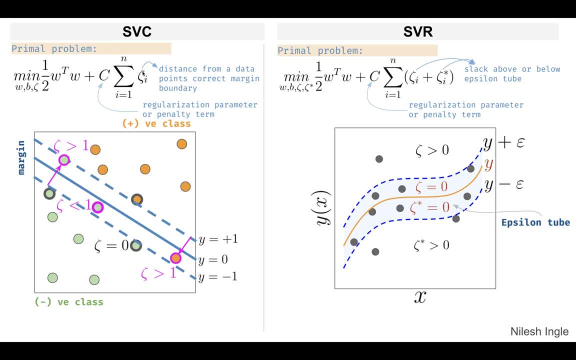 that we have seen before and that we have seen before. and here we have the regularization term, here we have the regularization term, here we have the regularization term with c and zeta, so zeta is again the with c and zeta, so zeta is again the. 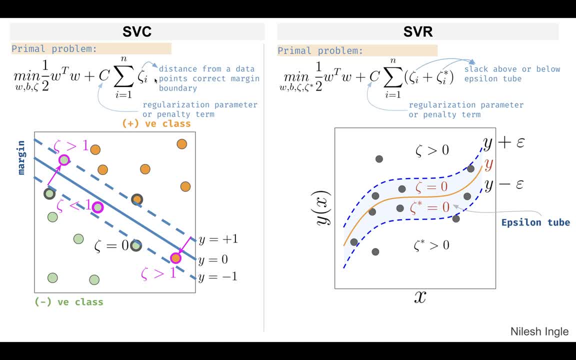 with c and zeta. so zeta is again the distance, distance. distance for how far they are from the decision, for how far they are from the decision, for how far they are from the decision. boundary, boundary, boundary, and then c is, and then c is, and then c is the regularization parameter that. 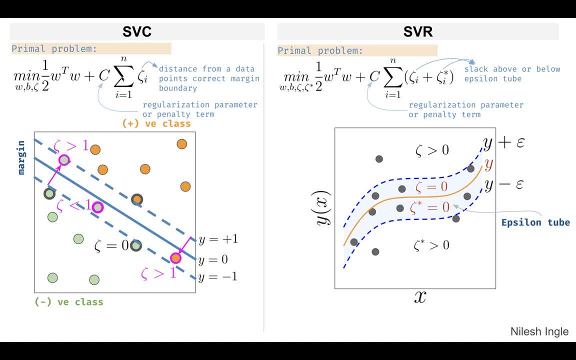 the regularization parameter that the regularization parameter that can be used to control, can be used to control, can be used to control how much penalty we put how much. how much penalty we put how much. how much penalty we put, how much penalty we allow. penalty we allow penalty we allow to be put on the misclassified data. 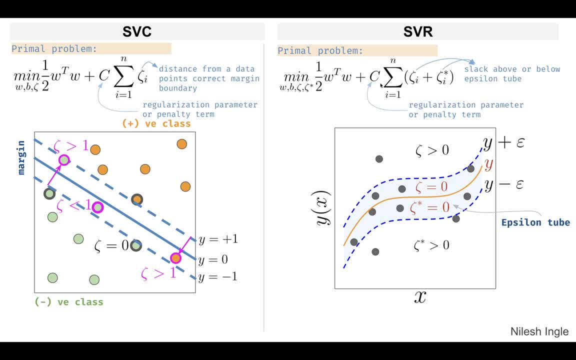 to be put on the misclassified data, to be put on the misclassified data: points, points, points and similarly. here we have the same and similarly. here we have the same and similarly. here we have the same setup, except that we instead of just one setup, except that we instead of just one. 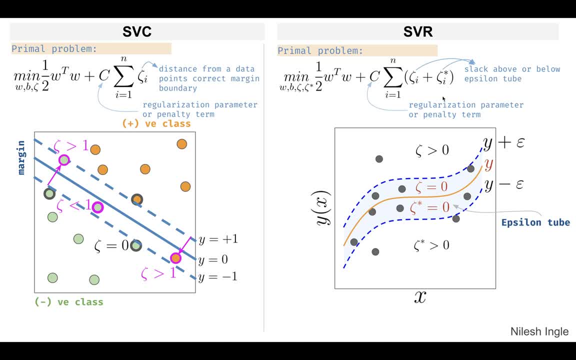 zeta. we have zeta i plus zeta star i, and that's because we are looking at the space above and below the epsilon tube, as shown in the figure below, whereas in case of the classification task, we have a different situation, where we are interested to keep things out of the margin. 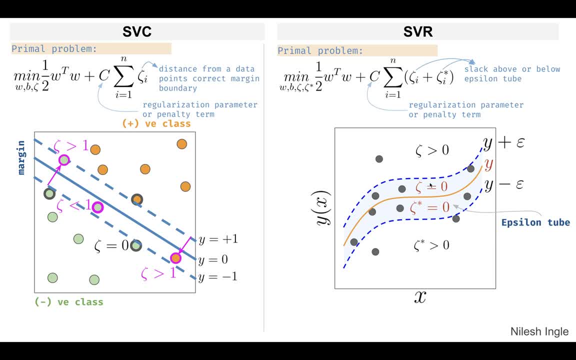 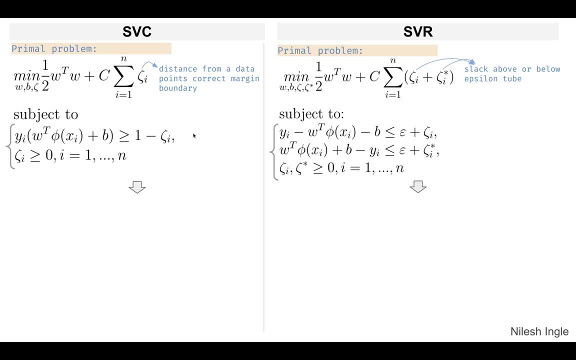 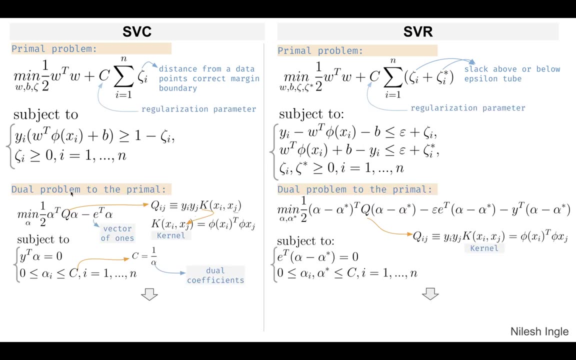 whereas in regression we want to keep things inside the margin. so that that's the difference there and these minimization equations are subject to these constraints that are shown here, and so that can be reduced to this particular minimization problem, which is: alpha transpose q of q, alpha minus e transpose alpha. so here the alpha is, the alpha represents. 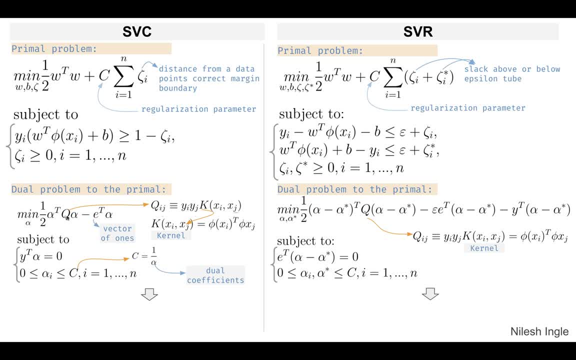 the dual coefficient, Student's y transpose alpha song conditions for the data points and the q is the kernel as shown here. and same thing on this side for regression, except that now we are getting taking a difference between alpha and alpha star and we have these additional terms on the right hand side for this minimization task. and 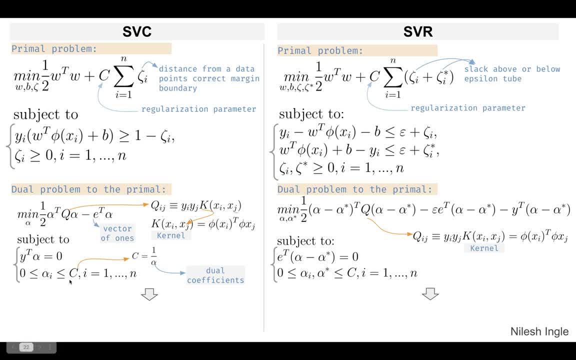 these again are subject to these conditions that are listed here, and the final decision function then looks like this: so where i is in support vector. so this is only this. for these calculations we are considering only support vectors, because the value of alpha for all non-support vectors. 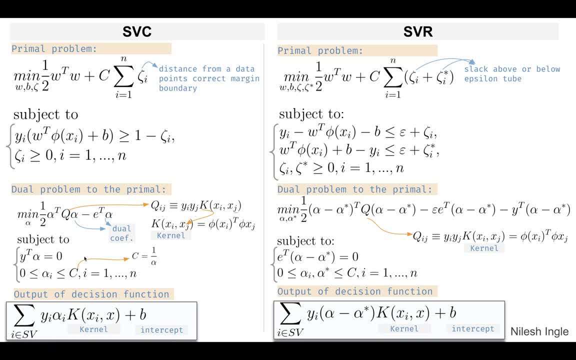 would be zero, and so that just makes the computation easier as well. so we have yi, alpha i, k, k of xi, x plus b, so b is the intercept, and we have the same equation on this side, except that we are taking a difference between alpha minus alpha. star in on, for when we 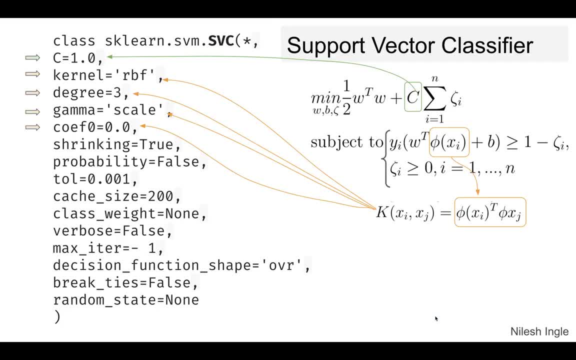 are talking about the regression and how then the values that we talked about can be tuned or tuned in sql learns method. so if we look at the support vector classifier method, svc- this is what you'll see. when you look at what parameters could be input into this particular method, then the c is the c that we have here. 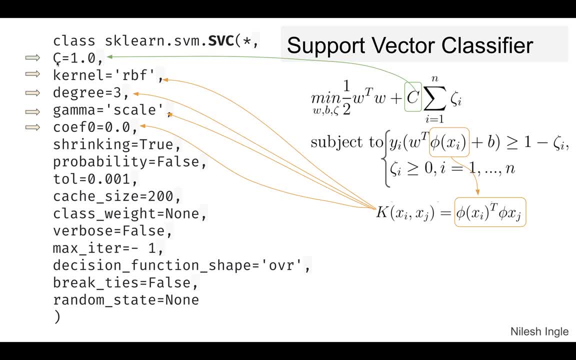 the regularization parameter so you can set a value for that. so if you are doing a grid search, cv or cross validation, you can put a range of these values to kind of change the width of the margin and then allow change the threshold of misclassification for each of those data points. 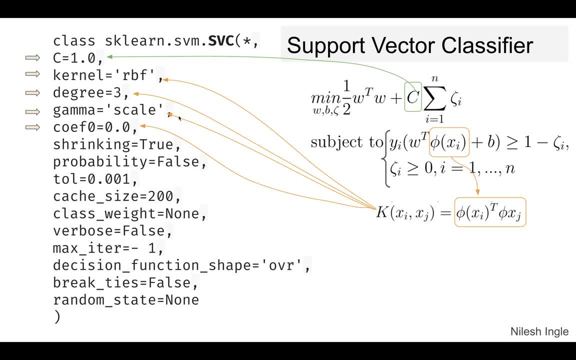 and then, additionally, with the kernel functionality, you can change the type of kernel. you can change if you select a polynomial kernel. you can change the degree. you can change the, also, again based on the type of kernel, you can change the gamma value. you can change the other type of the. 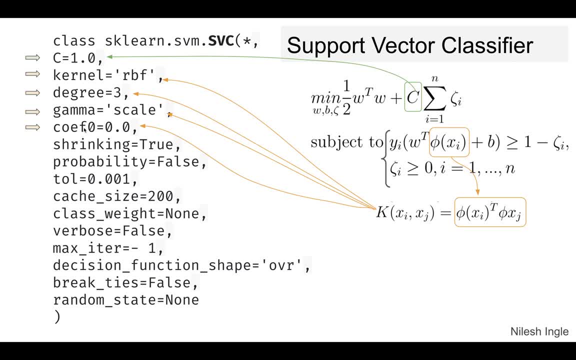 gamma value. you can change the other formula accordingly if you want. you can change the SPD id column or you. you now have what to change. so this is a pretty nice smartemon. change the coefficient. so all these functionalities allow kind of to fine tune the fit that you would. 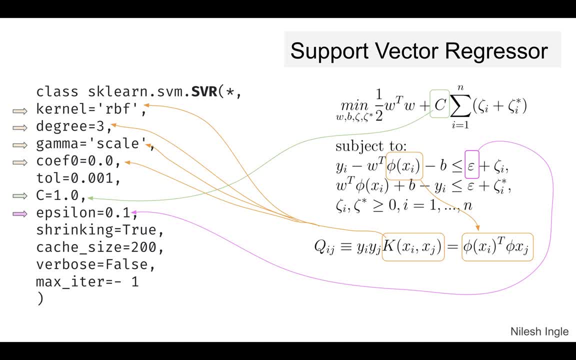 need for classifying a particular data set. similarly, for regression, we have similar functionalities as we have seen before, but here, in addition to that, we also have a value for epsilon that can be tuned. so with the value of epsilon we can, as you can, as you saw before, that would. 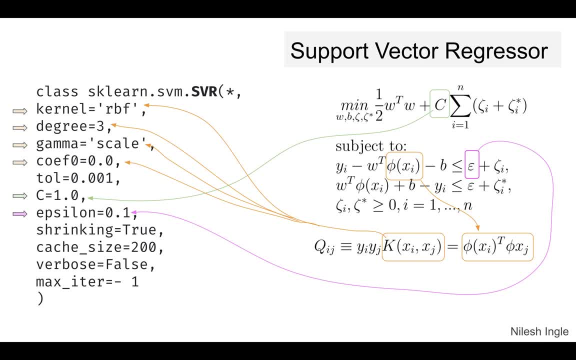 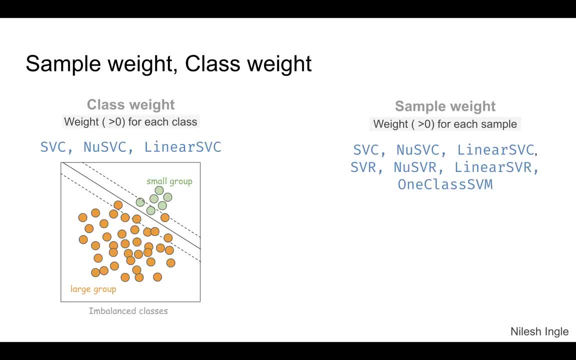 control the epsilon tube within within the fit and going further. there are additional functionalities that can be used, which is related to sample weight and class weight. so the class weight is as shown here, which is, let's say, we have two sets of data points- the orange data points here- and 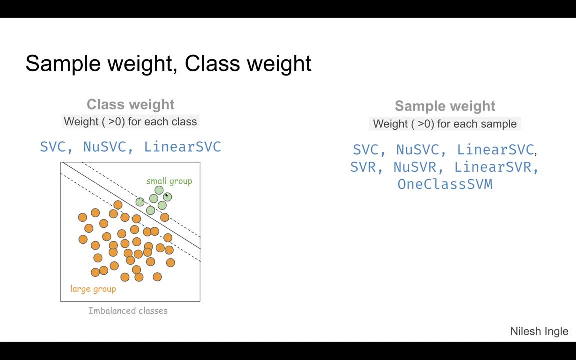 which are large majority, and there is, let's say, a very small number of or green data points that need to be classified. now here, if we with and without class weights, it could make a difference to get a correct decision boundary between those data points. you can see here that we have two sets of data points: the orange data points here and which are 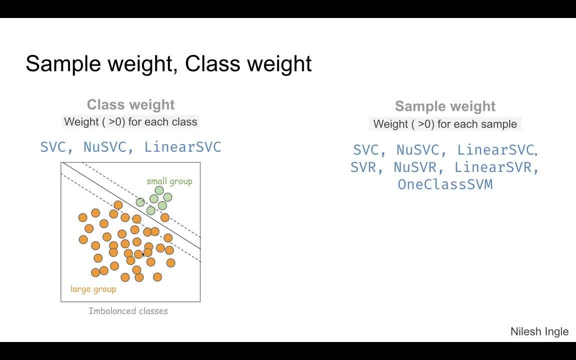 so what the class weight allows is, we can give a more, more or less weight depending on which class is a majority or minority in the data set, in addition to using class weight, and this can be given as a dictionary input when we are setting up the model- and sample weight is another version. 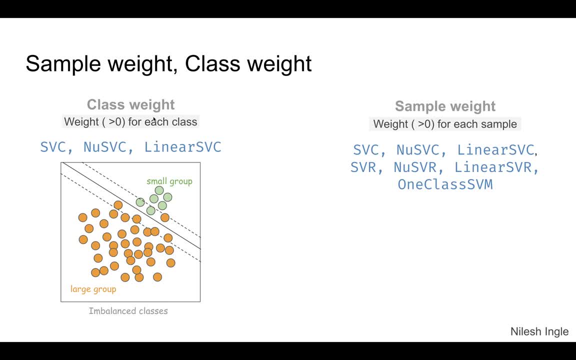 so instead of giving a weight for each class here, we are giving a weight for each class here. in case of sample weight, we can set a value for each sample or each row of the data set, and so then, each data set, each sample or each instance would have its own weight. that would be. 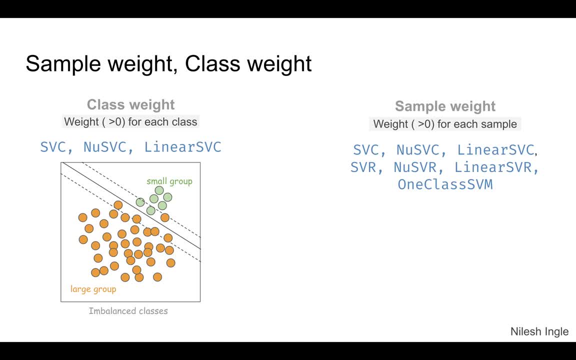 then used while performing the fit to find the optimal hyperplane that separates the class or finds the best regression fit and class weight is a all available for, of course, the classifier, so svc, new svc, linear svc and the sample weight is available for all these methods using. there is both classification methods as well as the. 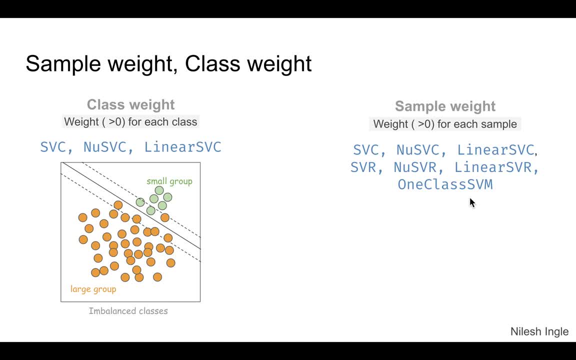 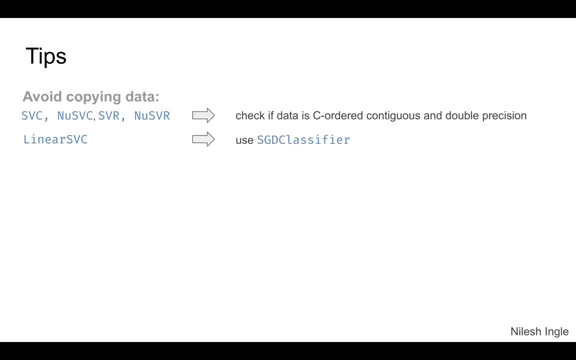 regression methods and also the one class, svm, that you could use to find the outliers. and here are some tips from the docs, major tips. there are more in the docs. if you want to read the labs here, go through. the one is to check if the input data is c ordered, continuous and so the 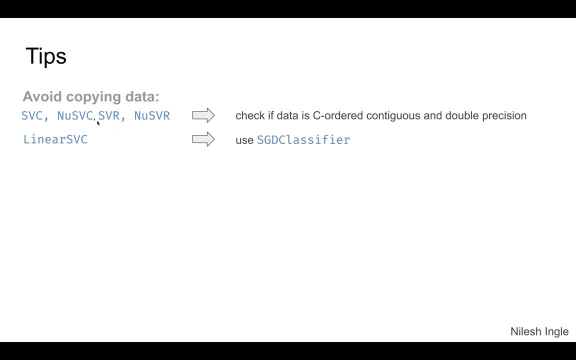 reason for that is: if it is not, then what is scikit-learn will do is create a copy of that, and so creating that copy is going to take much larger space if the data set is a much larger, and so you don't want that. what we want to make sure is check if 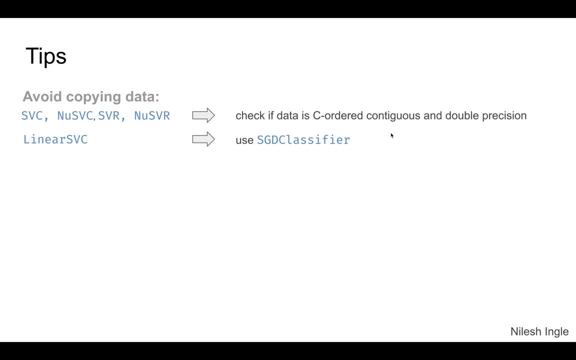 is c ordered contagious. forgot to put how to do that. the there is command in numpy that can do that. next, depending on what type of hardware you're using, the ram size could be changed for cache. so if you have more ram then you could change set the value for cache size to be higher. 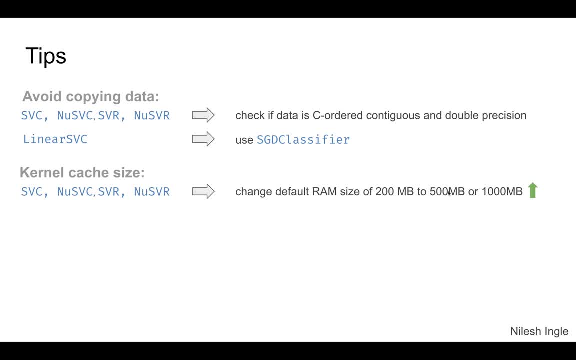 and so that could expedite the fitting process, the value of c, if you, if the data is noisy data, then what you could do is add more regularization and so you could decrease the value of c. that is, you're reducing the width or reducing the margin, and so it's the tolerance is. 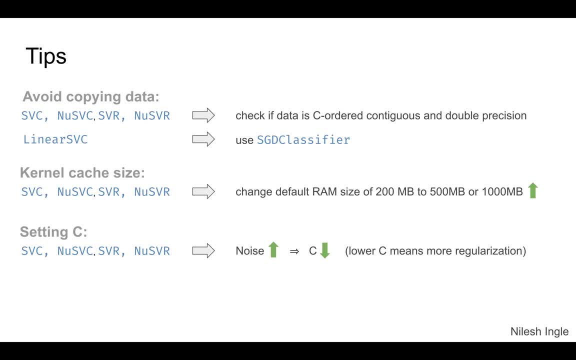 a lesser tolerance when we are trying to classify the data points and very important when working with support vector classifier support vector machines. you definitely want to scale the data so that the data is either between zero and one or minus one and plus one. that's very important. 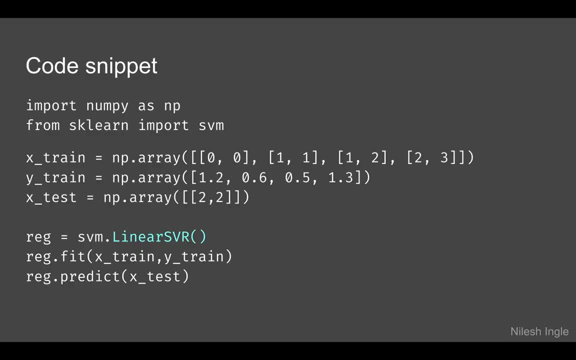 and finally, here is a code snippet, uh, which is standard. i have the data set and if you are using a regressor such as linear svor, then create a variable reg, fit it on trendset and then call it for prediction on a test set. so that was it for this video. i hope in this video you got an intuition about 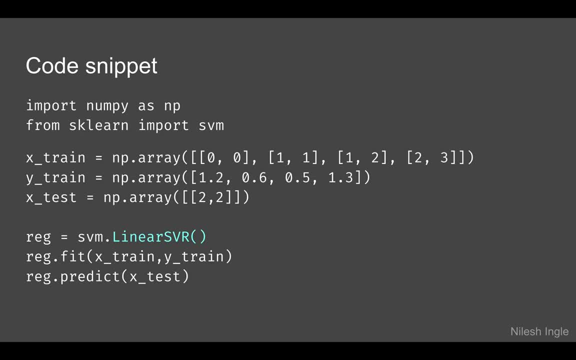 what support vector machine is and how it can be used for the tasks such as classification or regression. and we talked about kernels. if you need more intuition about how kernels work, so just checking out the videos, think on the fifth video, before this particular video and in the next.